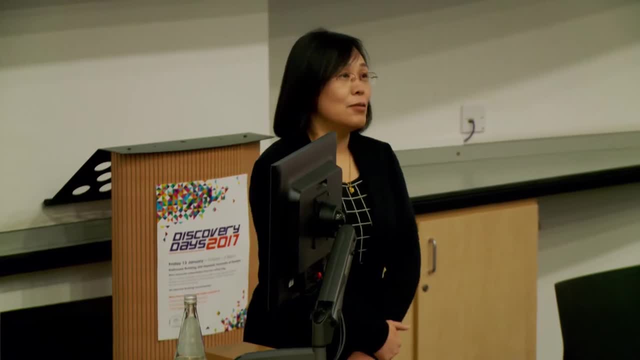 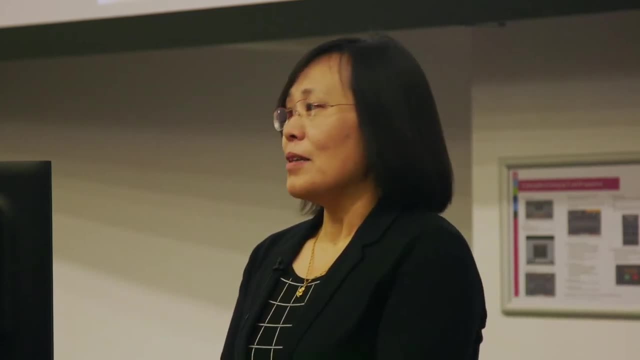 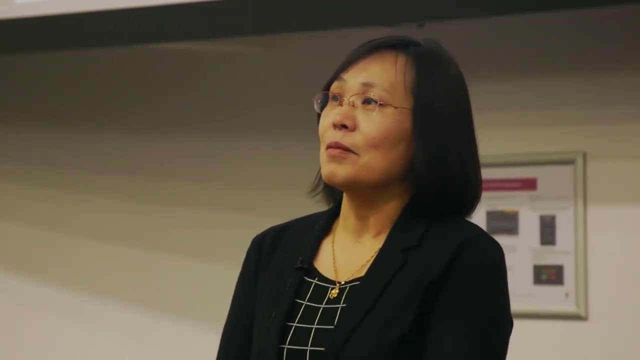 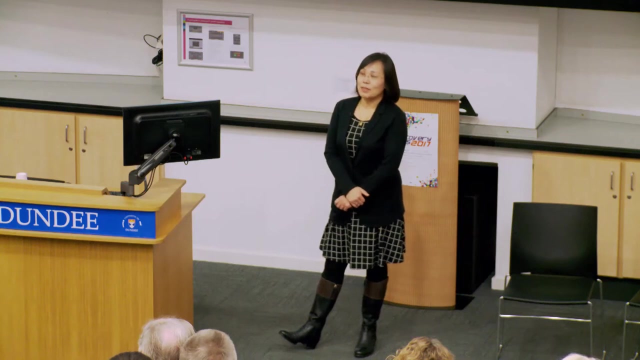 Dundee to study on ultrasound and also teaching students for ultrasound topics there, Because ultrasound is quite important for medical care, and to look at ultrasound. actually that's my starting point of the research in Dundee: Looking at ultrasound. people thinking about ultrasound probably were thinking about ultrasound imaging. 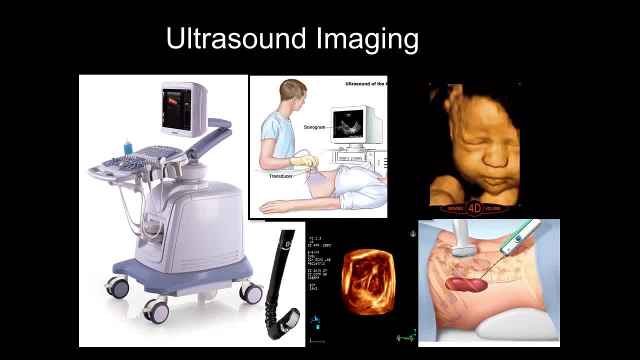 Ultrasound imaging probably is widely used in healthcare and ultrasound imaging systems actually looks like that Probably lots of people. if you've been to the hospital you will see that it's the system over here and it has a monitor system on the top to show the images there. 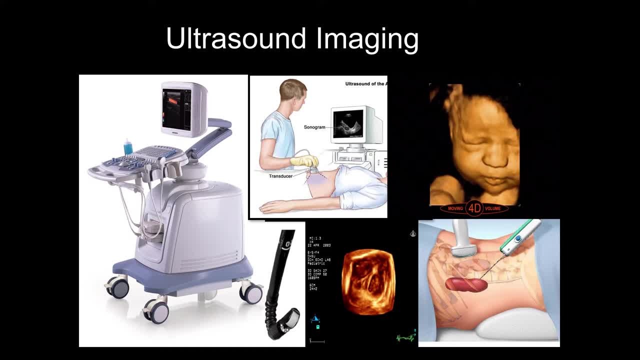 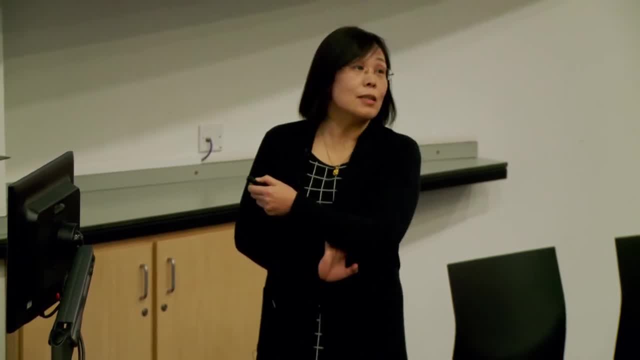 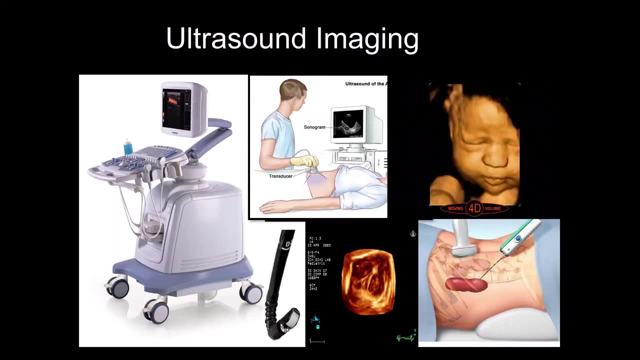 and also they have a control system. Also, there's a very important device over here that's called transducers, which is in touch with the patients so that we can receive some signals, to have the images there. median and ultrasoundид- minimal ultrasound營. 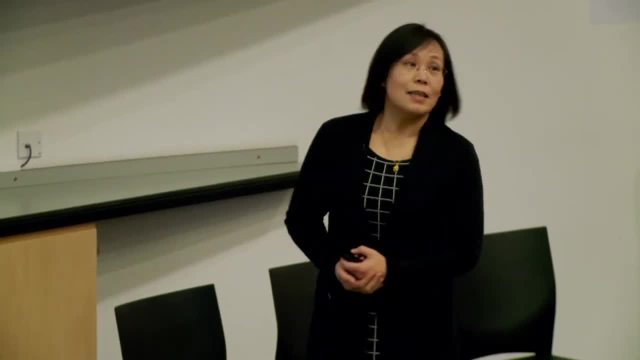 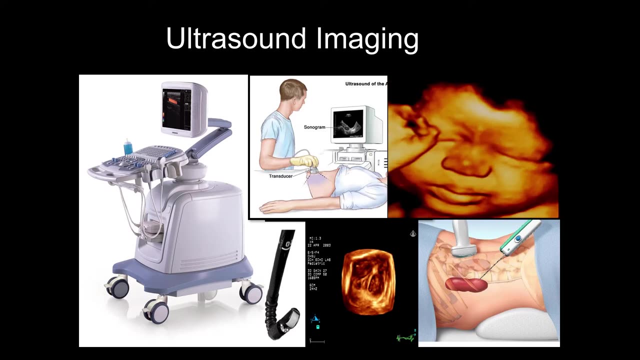 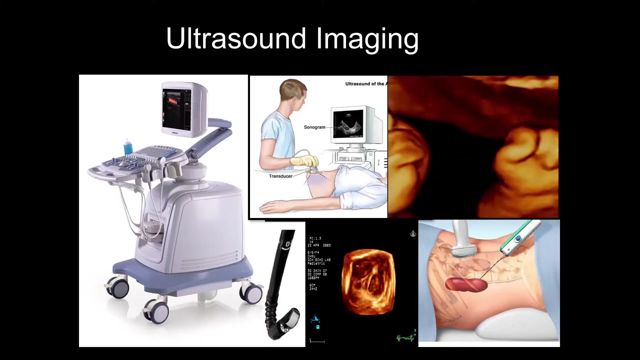 infrared digital也 fi. lots of new advantages and development there from the 2D scans and the black and white image there and into 3Ds now in 4Ds and you can see there is the ultrasound image is quite clearly showing the baby movements in and they are so quite nice fixtures over there and also ultrasound. 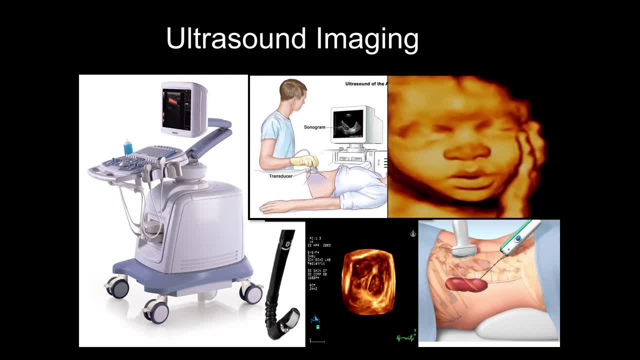 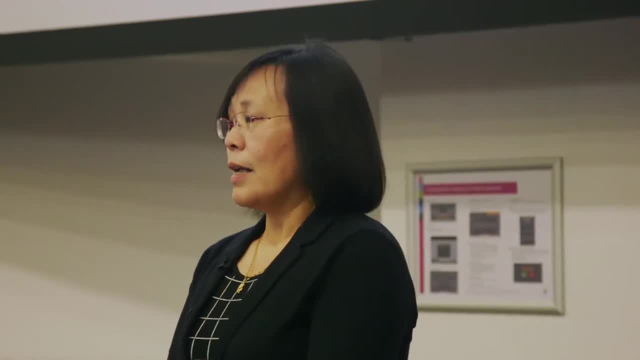 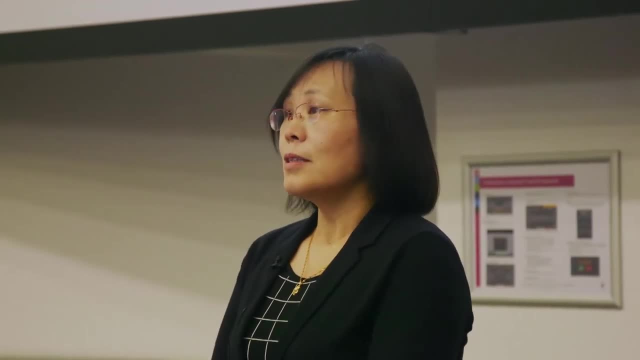 has been used, not only just scanning for babies, have used for many other applications there, for example, and ultrasound has been put under the endoscopies there to scan the inside of the bodies. and also, importantly, there's ultrasound has been used as an image guidance for many procedures. 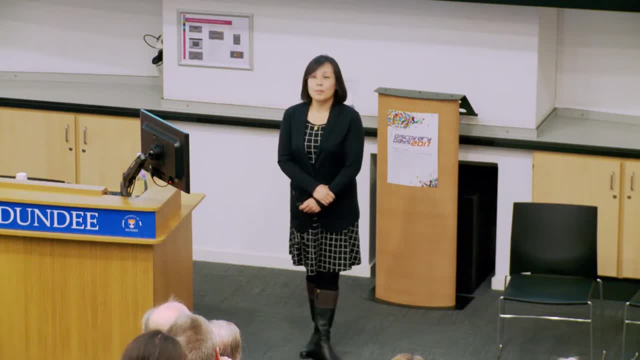 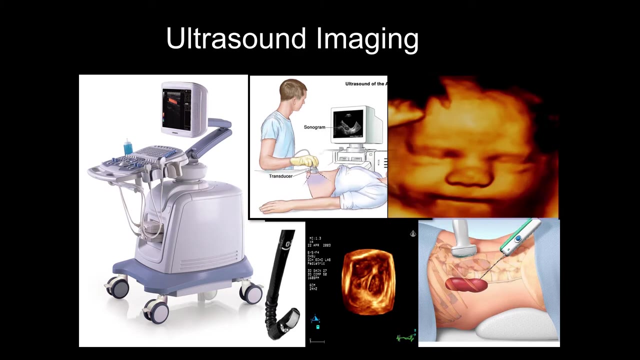 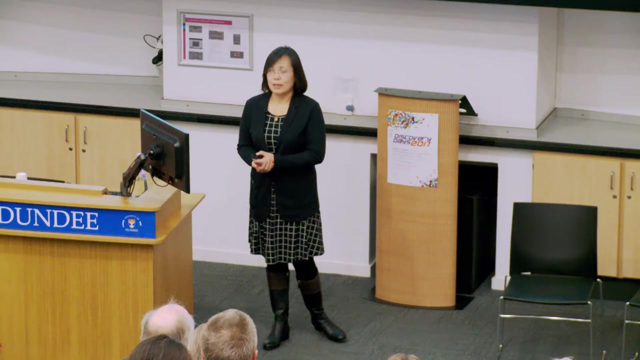 for example, and when people doing the biopsies procedures there there's often is done under ultrasound guidance, and ultrasound image has provided as a very important guidance for many procedures you know and also I'm going to talk about in the next few slides, talking about ultrasound for other applications. there ultrasound imaging is just like a sound wave. 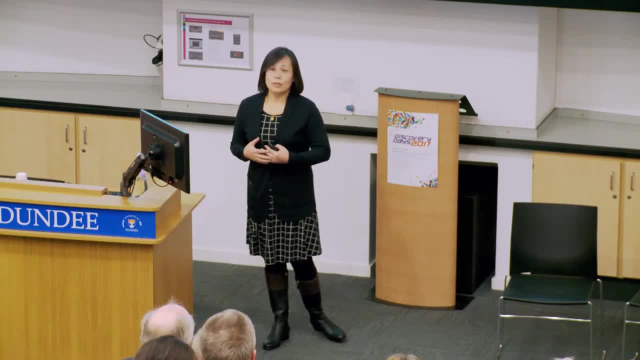 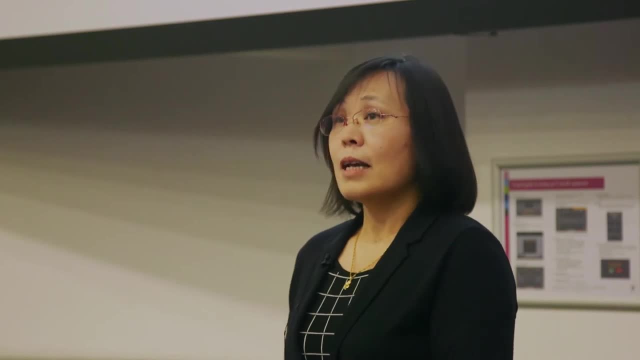 travel inside of the body and we, using the transducer, we can receive some signals and to provide an image and to guide the procedure there. and this has been used as a very important tools for diagnosis as well, because of the development in ultrasound, they not only just see the image and they also can measure the properties. 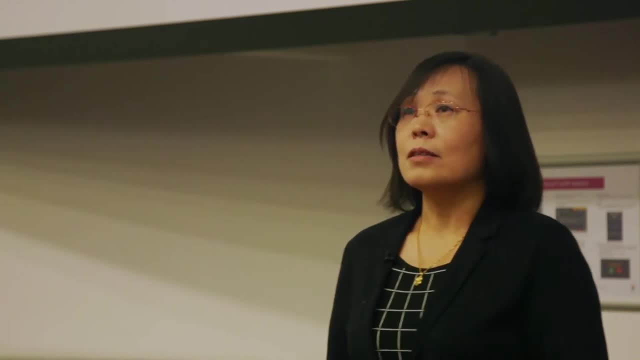 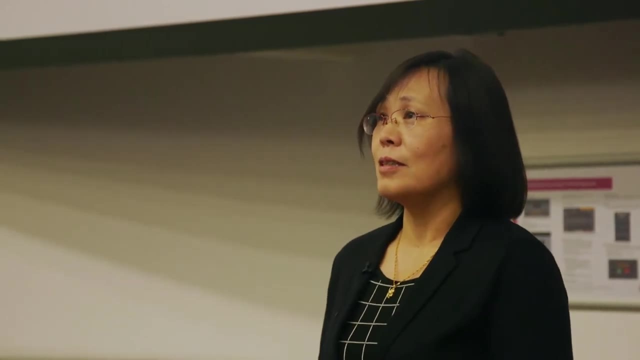 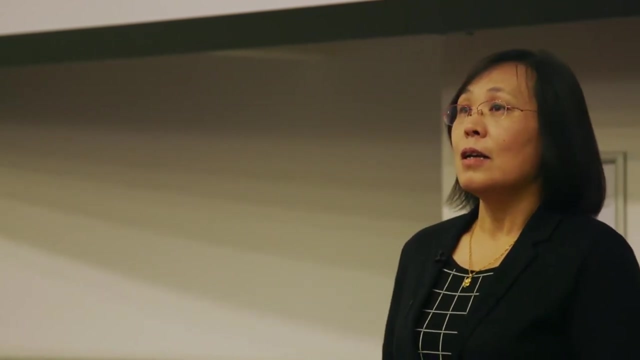 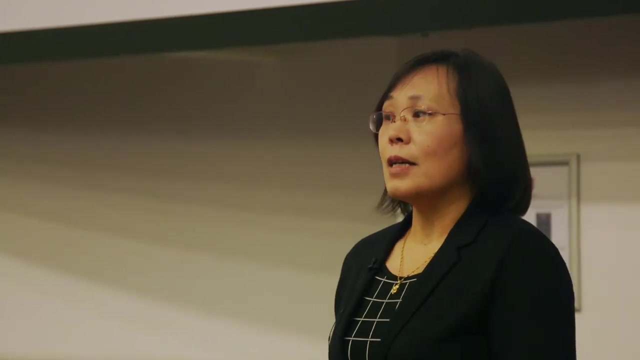 of the tissues as well. in other areas of ultrasound probably people probably not know and that many knows about, ultrasound has been used for surgeries as well. so in the surgeries, in the open of the keyhole surgery, is there people using the surgeons, using the ultrasound to dissect the tissues and how it works. 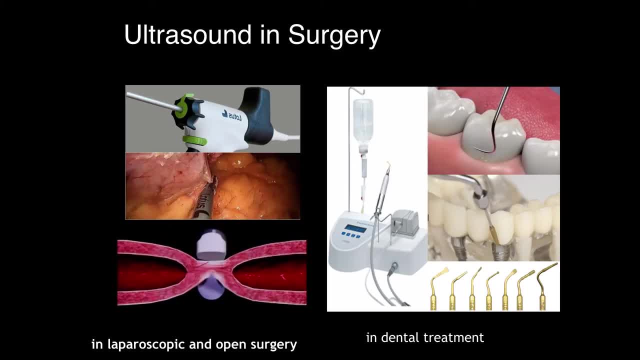 is that actually it's just using ultrasound waves or we say that as a mechanical engineer? we say that it's a vibrations motions, using vibrations motions to cut tissues to reduce the damage and reduce the bleedings. and also it has been used for other places. you know, if you go to the dental 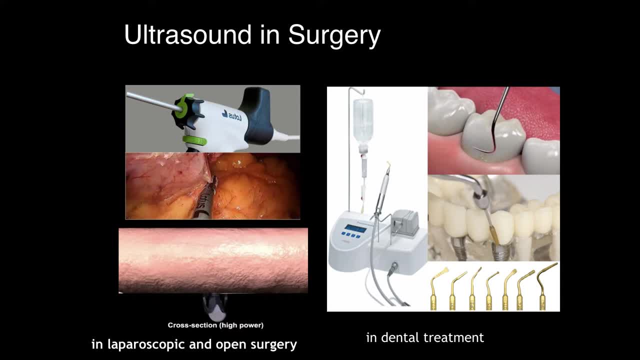 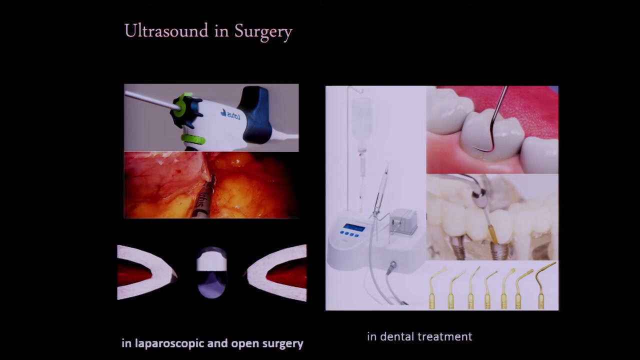 treatments there. you probably you have used ultrasound machines already. ultrasound has been used for dental cleaning procedures or the implant procedures there. because of the loss of different treatment there, as engineering we have to design different tools to fit for the different purposes there. so you probably will see that in the dental treatment rooms there. 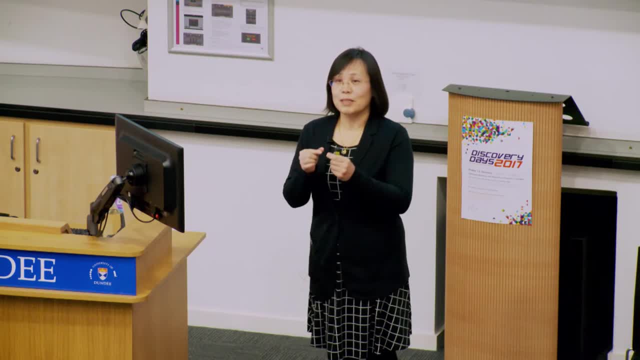 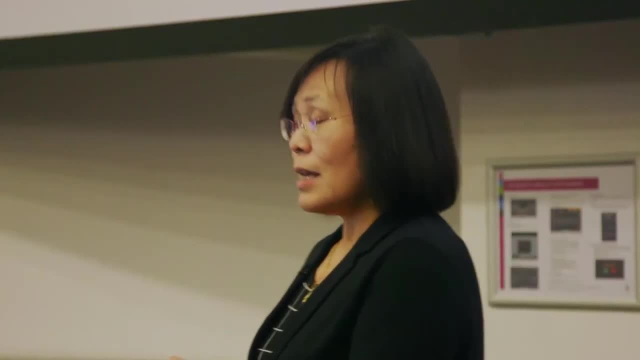 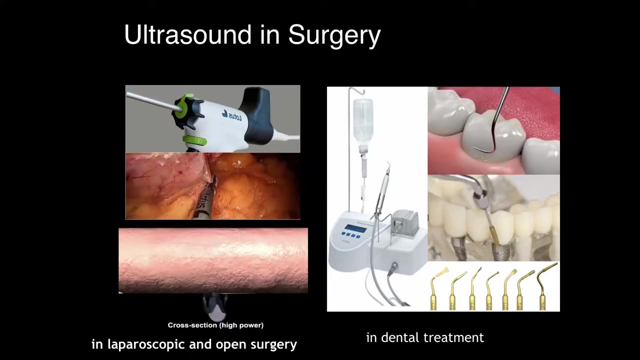 there's a lot of different types of the tooth tips and how to fit it to results, the device and for the different purpose of the treatments there. so the the key areas we do look in, as the here is the transducer here and that's provide a mechanical vibrations to the two tips. 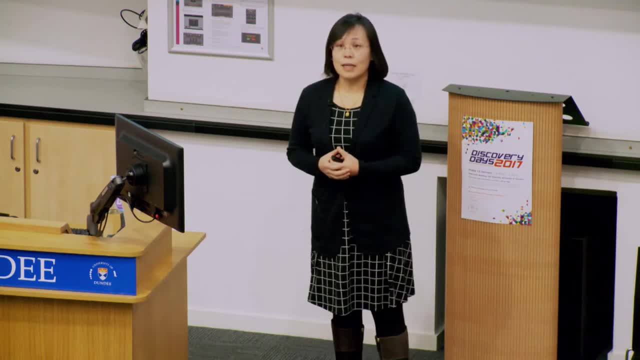 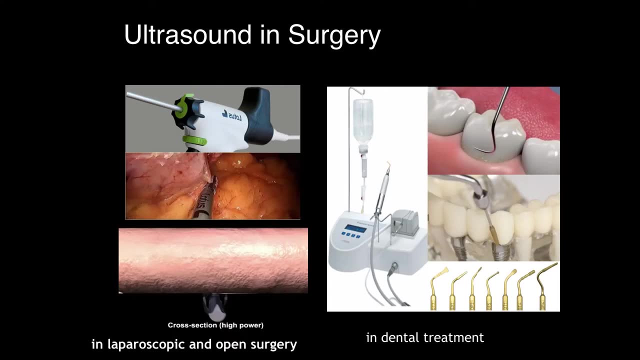 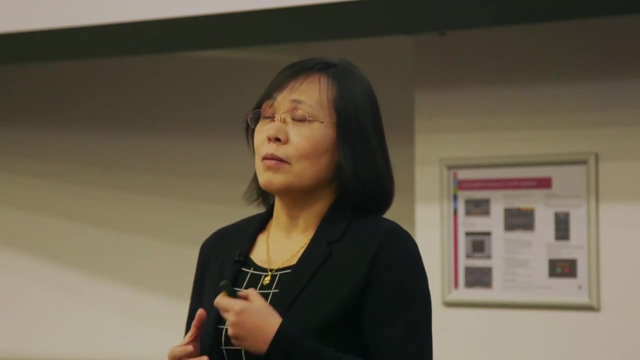 and applying for the different procedures there and for this case there, ultrasound has been used as energy source to provide a loss of energy, mechanical vibration and energy towards the, towards the surgeries, and to damage the tissues here, and the energy source and they provide over here is used of much higher energy but lower frequencies. here, then another one. 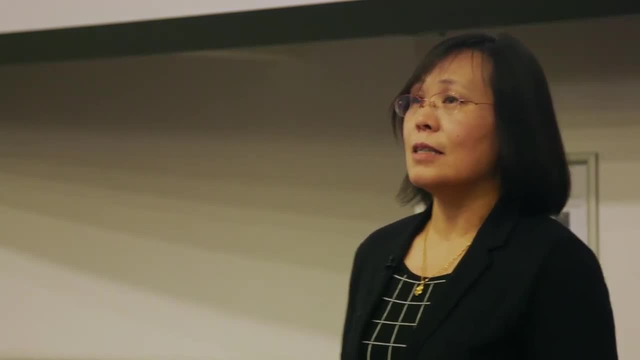 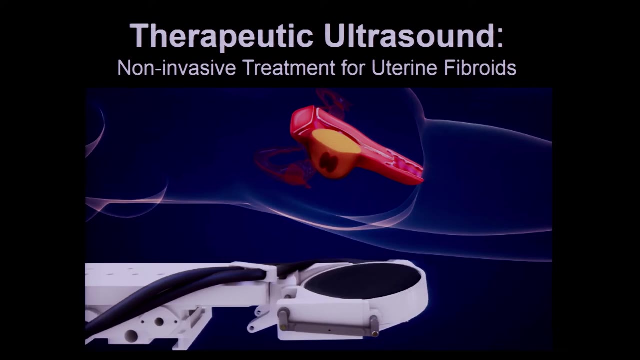 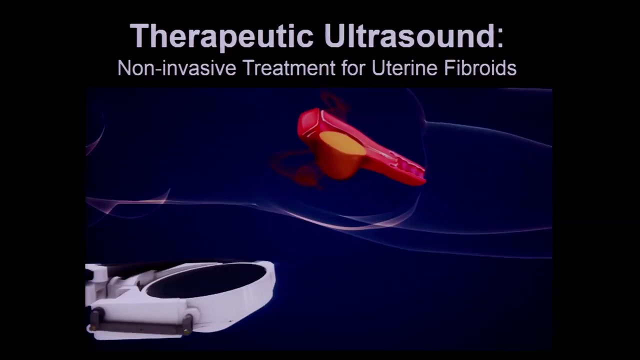 is very interesting. one recent in the recent years is developed as a using ultrasound for the non-invasive surgeries. so it's it's called that therapeutic ultrasound, using the ultrasound wave and focus inside of the body towards the tumors. if there's a tumor inside of the body without open. 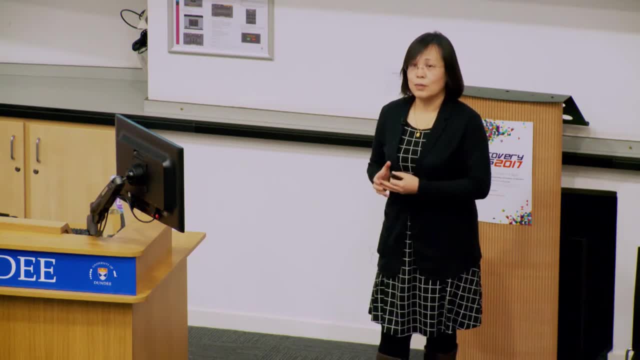 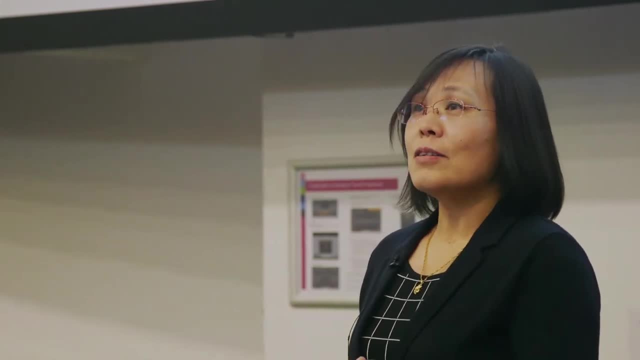 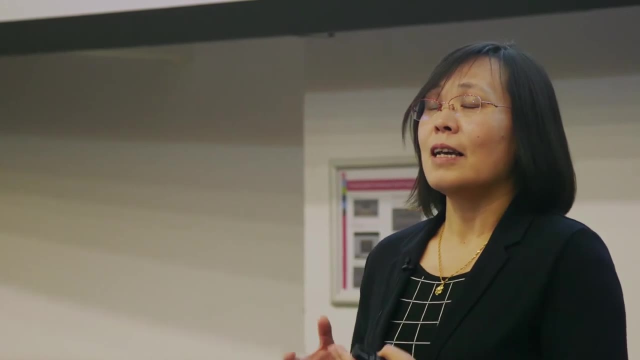 surgeries and you can treat tumors because of the energy put into the focus point there. instead of and open the surgery, cut the tumor out. so there's a new area to look at that the design of that kind of the ultrasound devices is similar to the ultrasound imaging devices and, using the 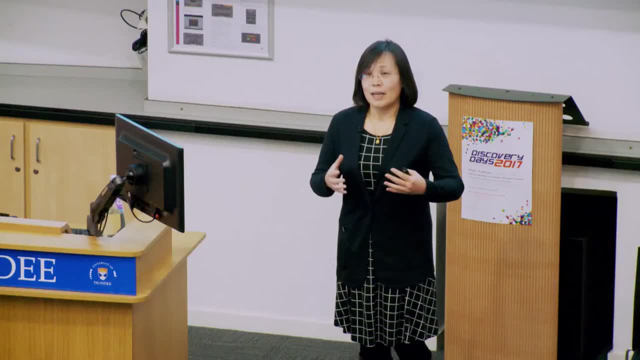 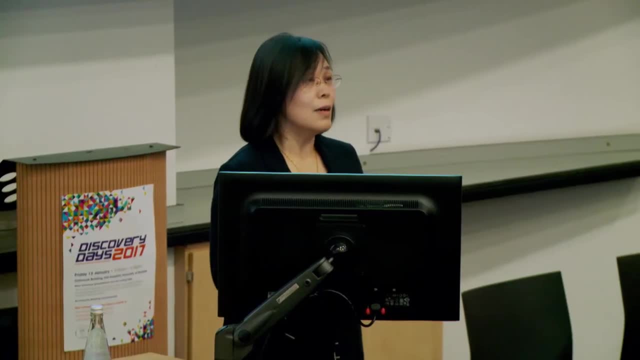 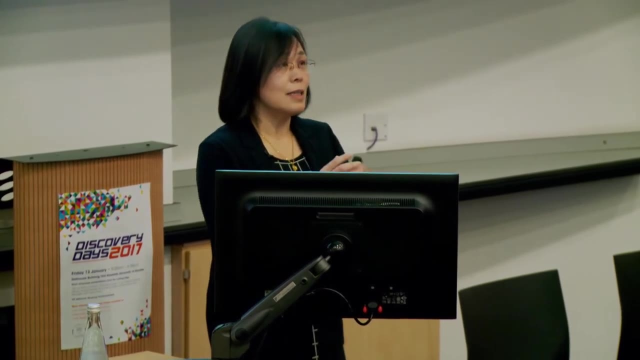 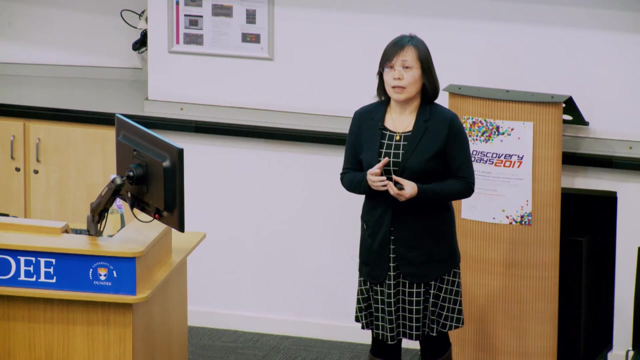 ultrasound energy, a bit of more energy, and apply to the, to the human tissues there and without focus, and there's quite harmless because the energy is not high enough to damage the tissue. but one is focus is generate massive heat around the tissue, around the tissue, the tissue you want to destroy. for example, it's a tumour over there. So 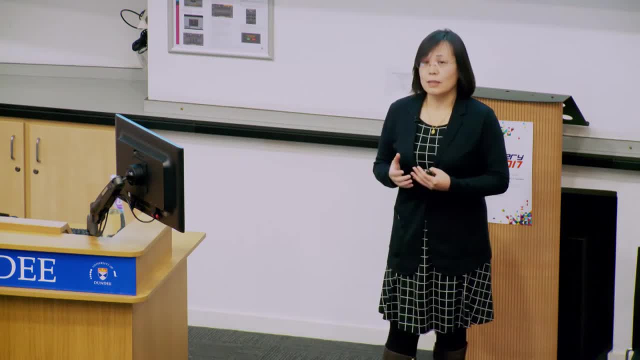 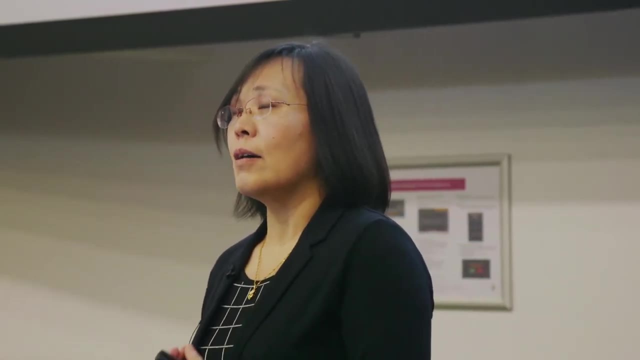 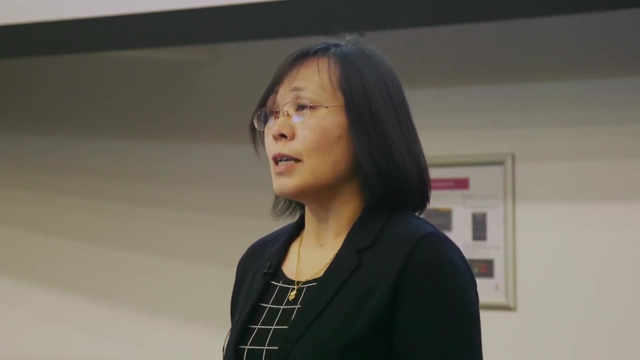 without a patient open, you can treat patients and patients can walk out from the surgery rooms. So that's one of the very interesting areas, a new areas for the surgeries, and it has been applied to many, many of the treatments there. For example, there's a liver and cancer treatments and prostate. 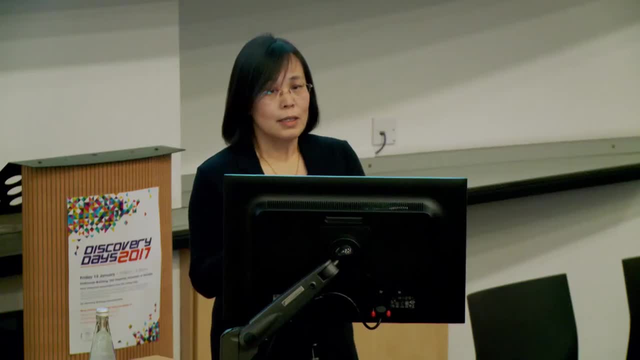 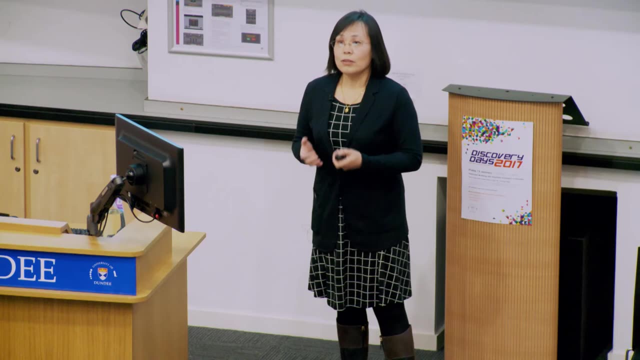 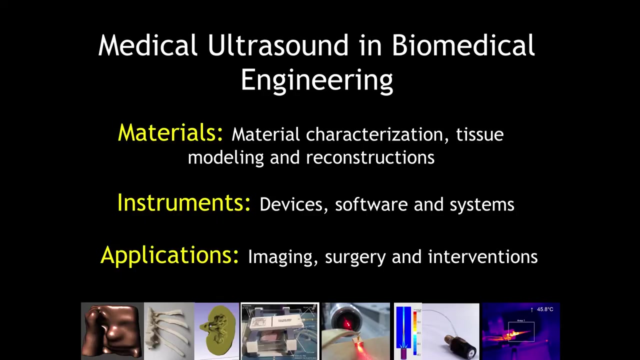 and brain tumours or uterine fibres are very common and treatment for using ultrasound right now. So there's a lot of interesting procedures and applications in medicine using ultrasound. but for us, if we want to develop further for ultrasound in terms of biomedical engineering, 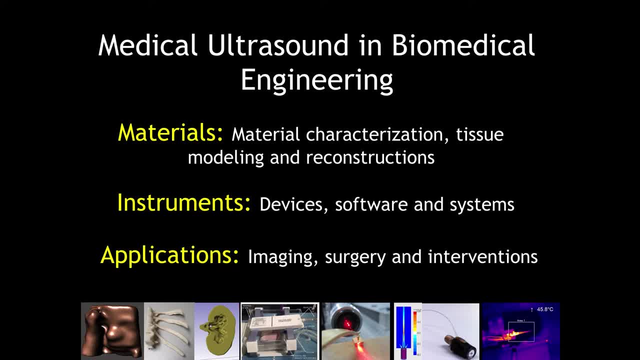 ultrasound research for us is what we're trying to do. is recruitment quicker than every other procedure for us, even when we, right now, We're using our knowledge trying to understand what happens between the tissues and the ultrasound devices and trying to find a solution to solve the problems? 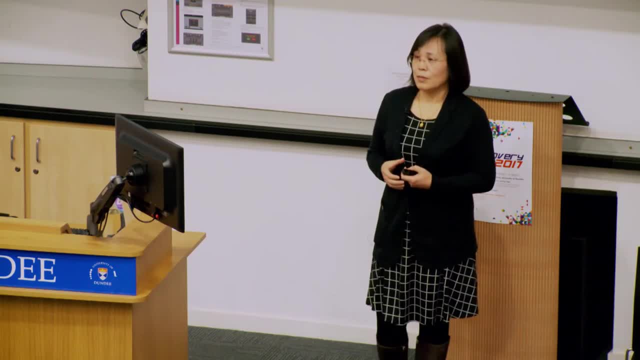 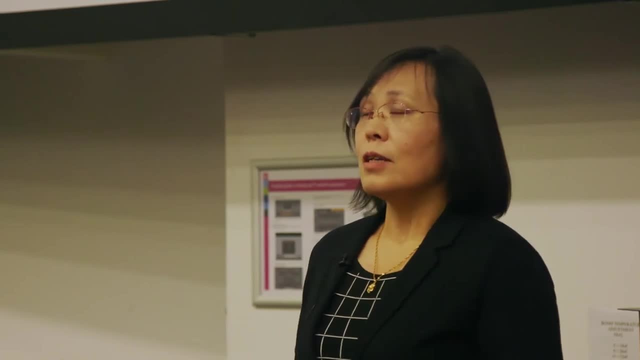 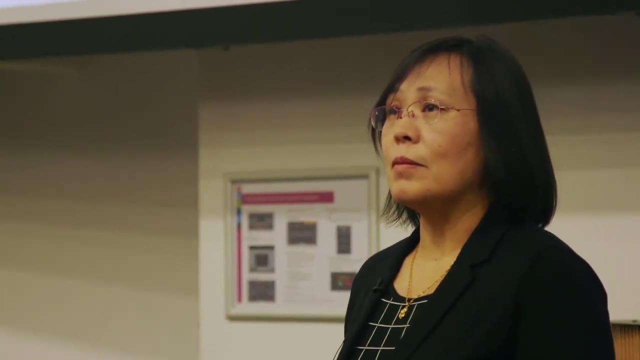 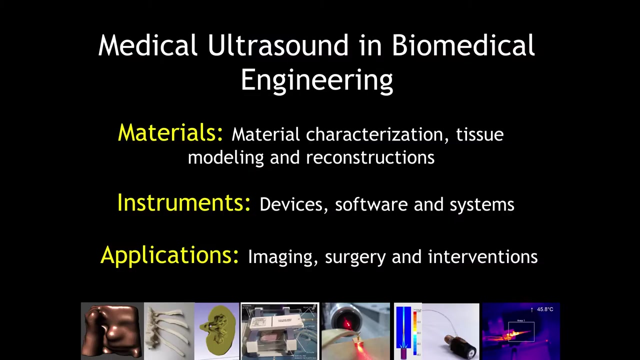 So in our research- ultrasound research- in our labs over here we set up very nice facilities to study tissues and to regenerate models for the human bodies, For example. we're using the data as we come from the ultrasound image or MRI image or CT image, we reconstruct it and trying to understand the structure of that and also 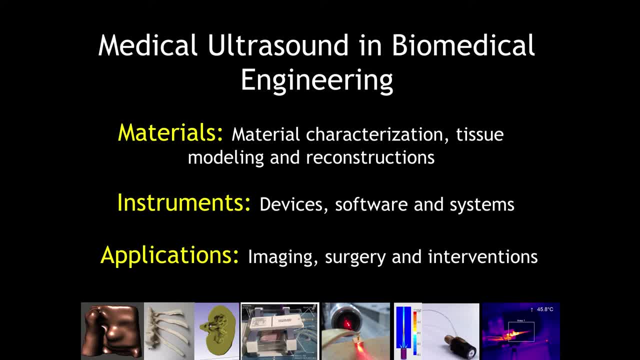 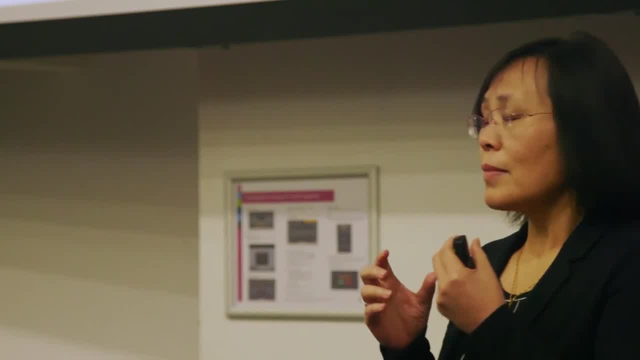 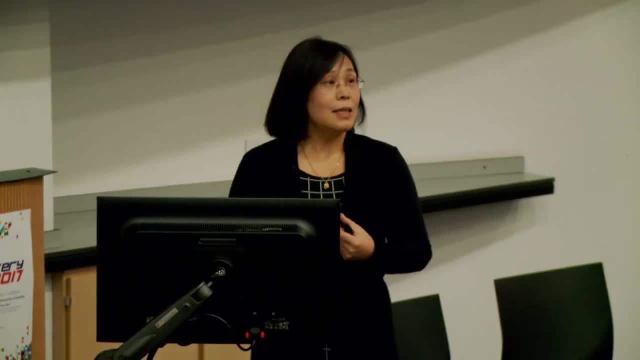 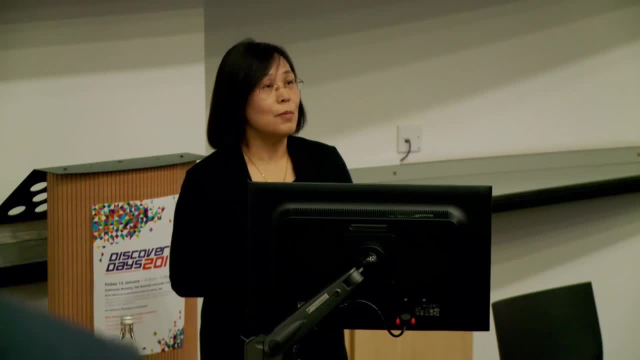 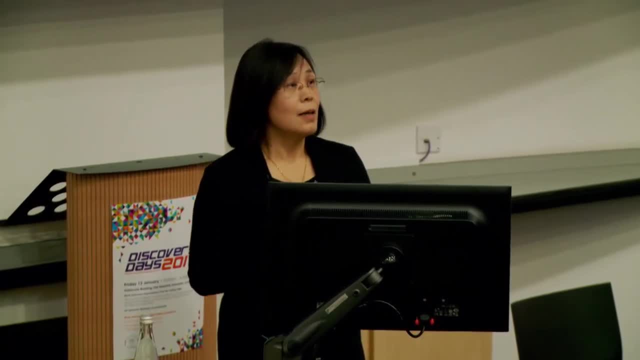 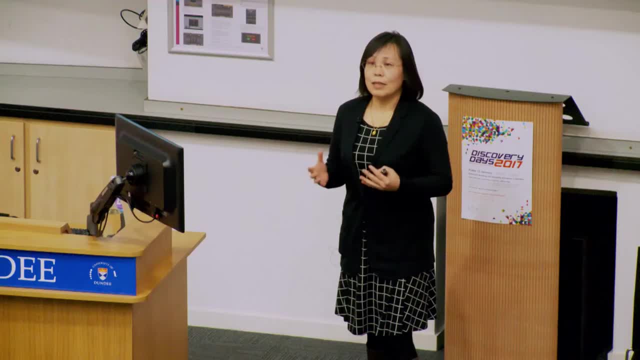 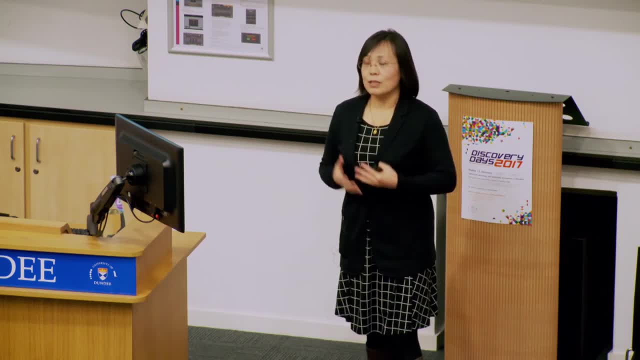 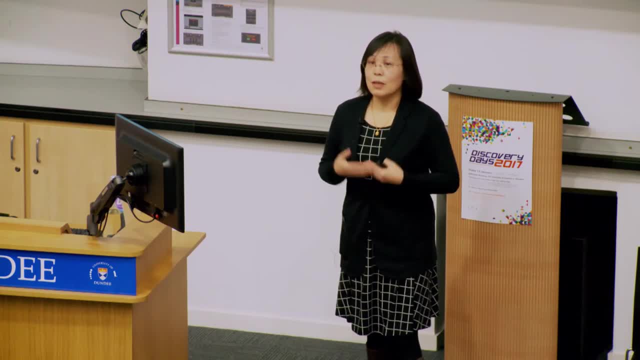 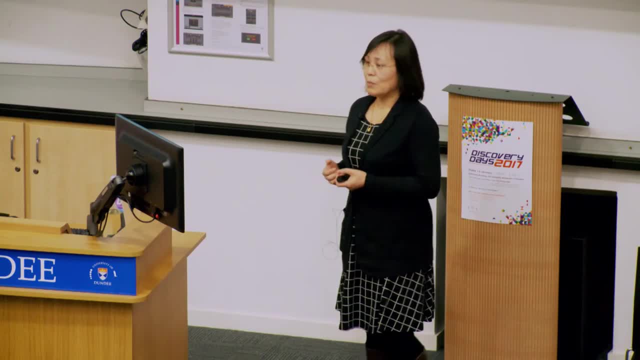 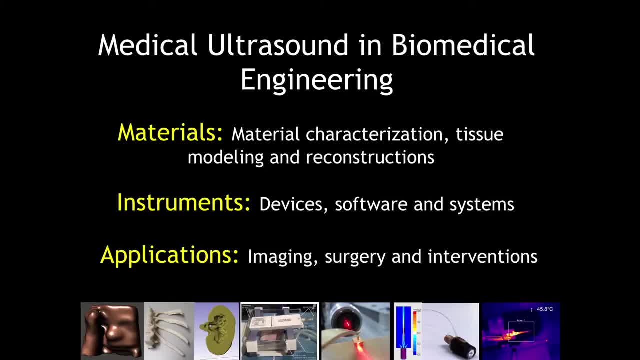 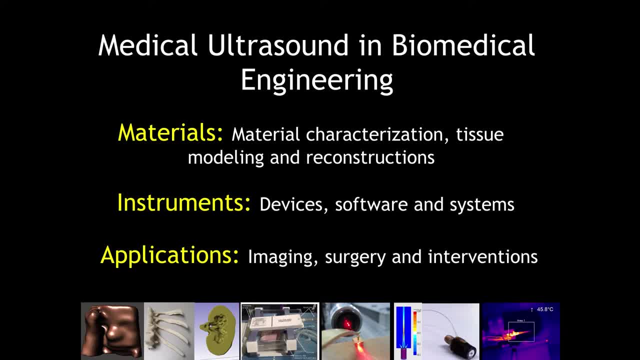 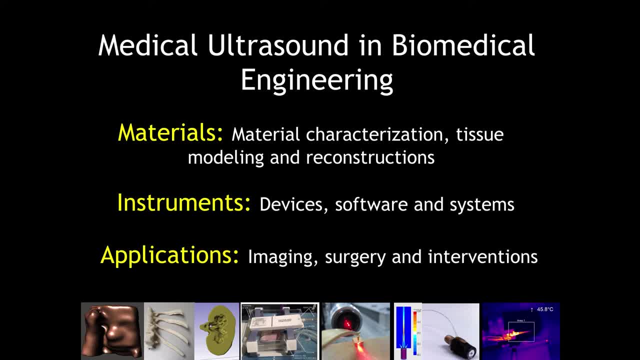 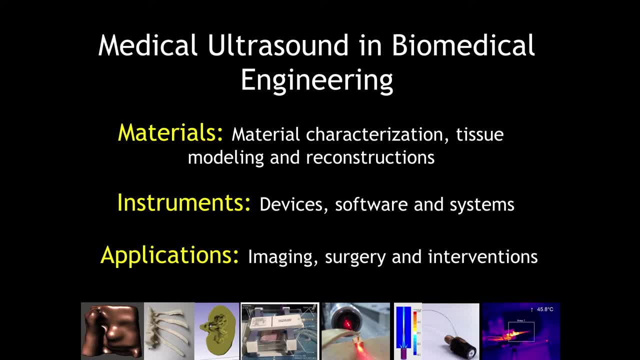 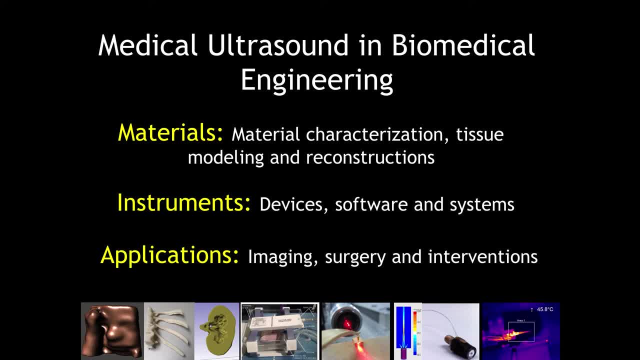 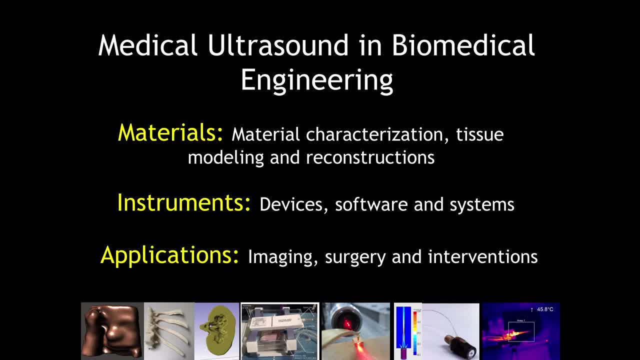 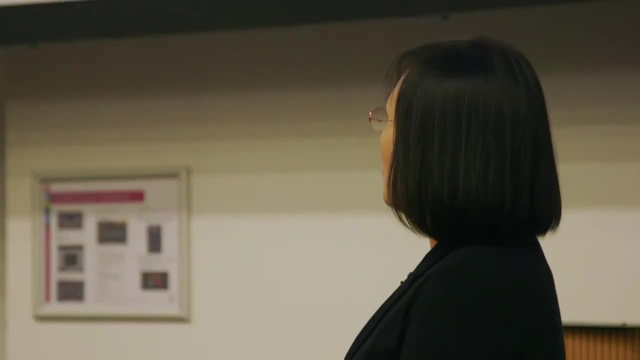 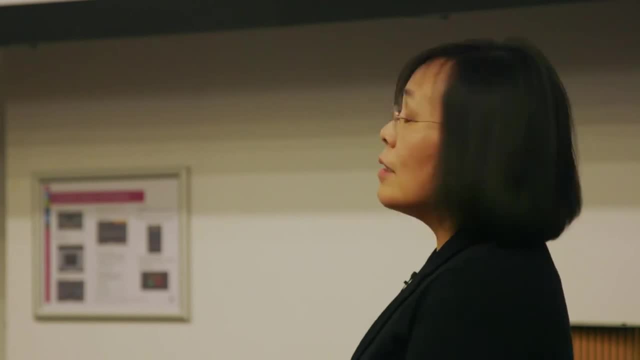 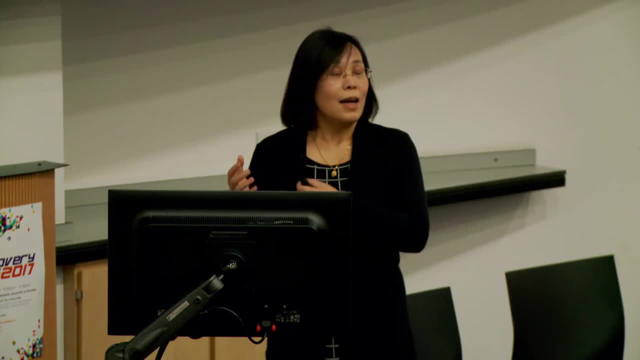 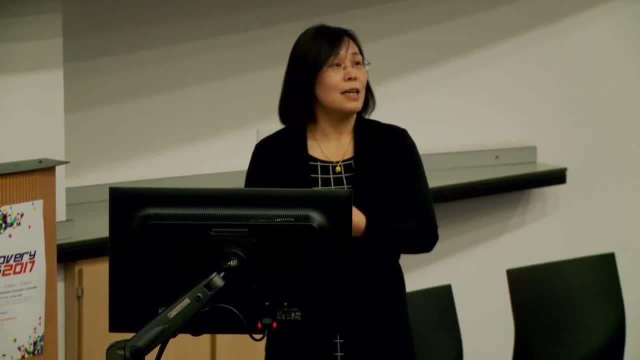 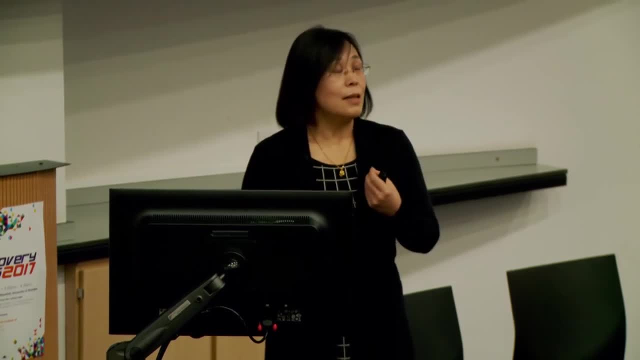 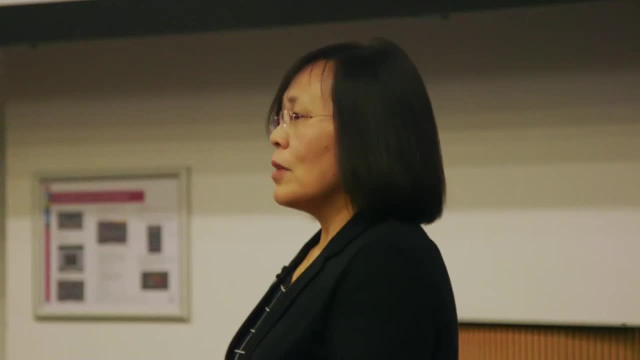 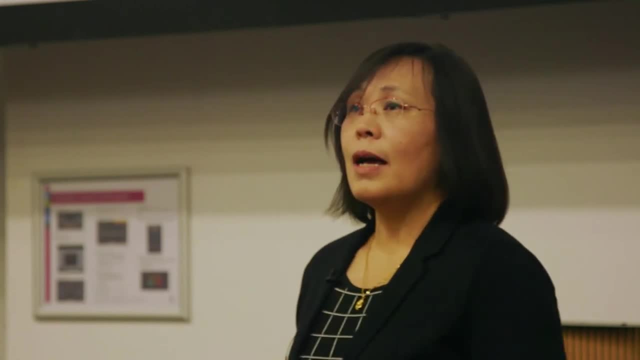 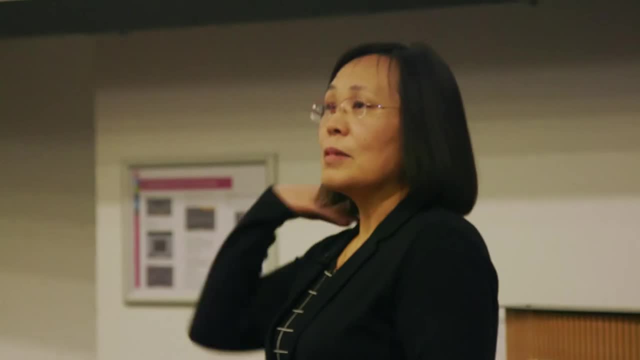 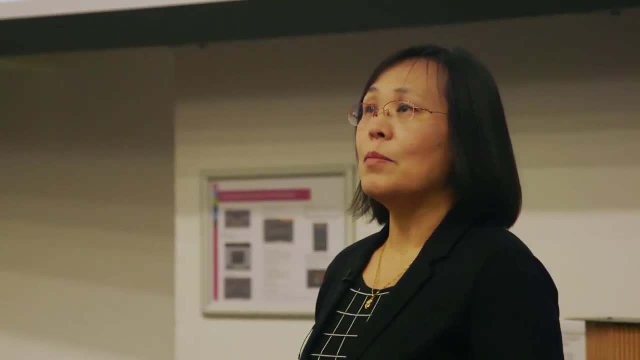 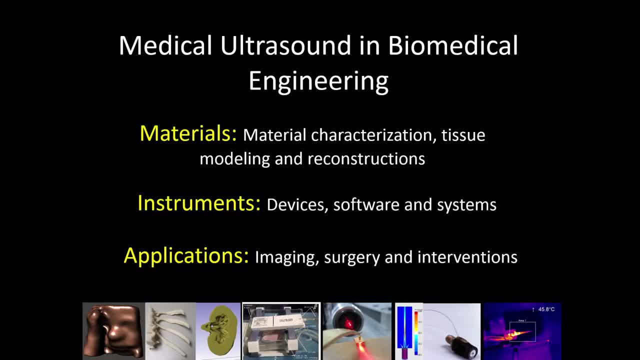 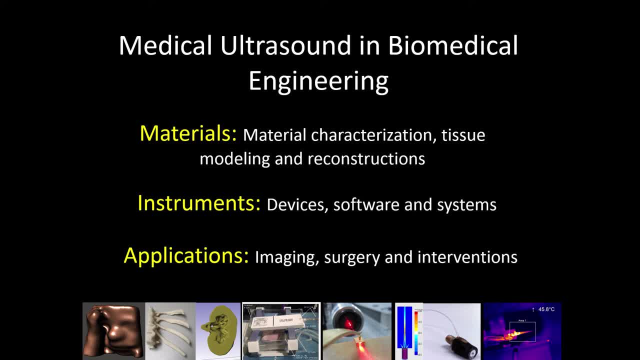 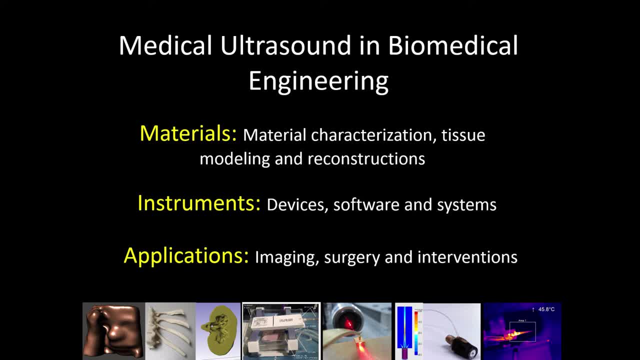 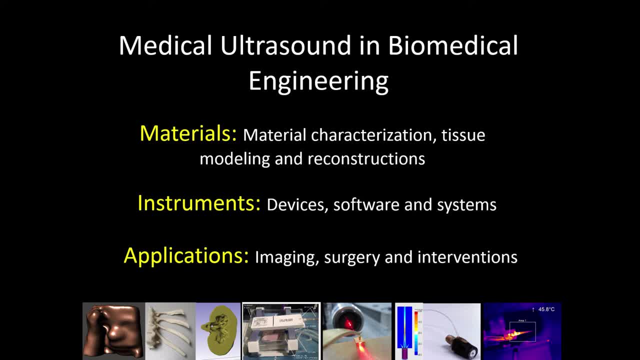 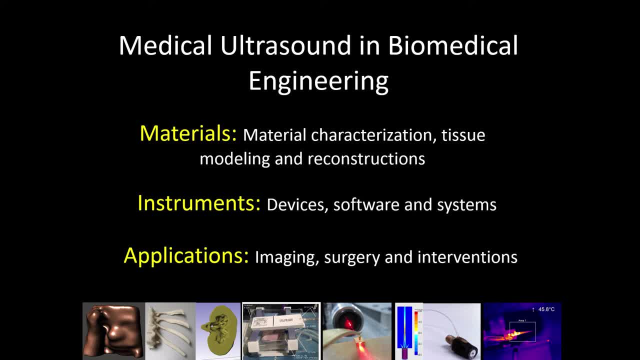 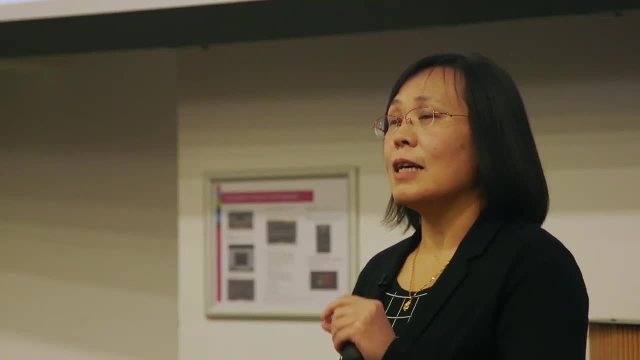 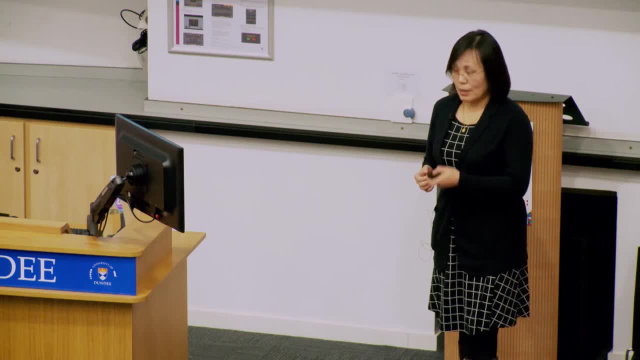 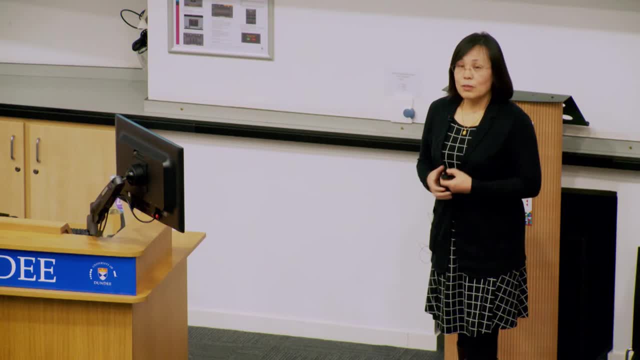 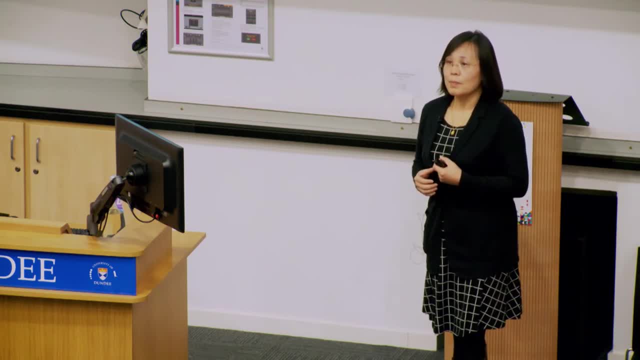 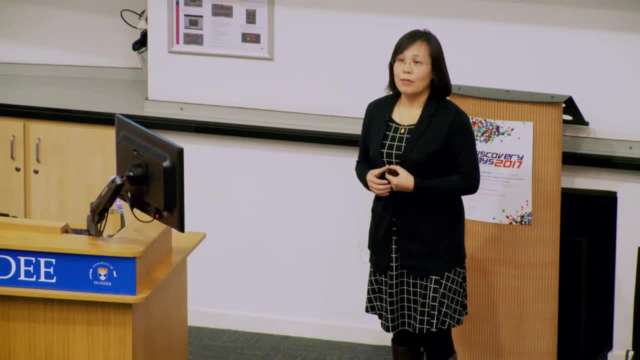 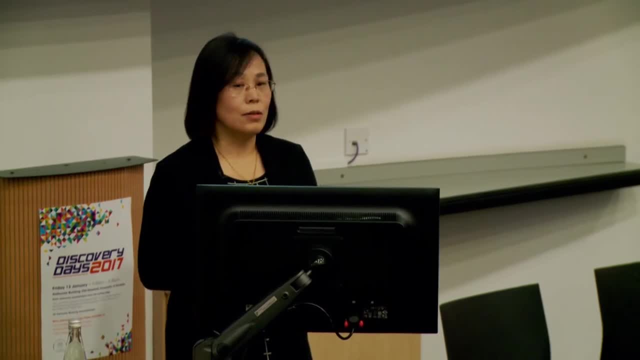 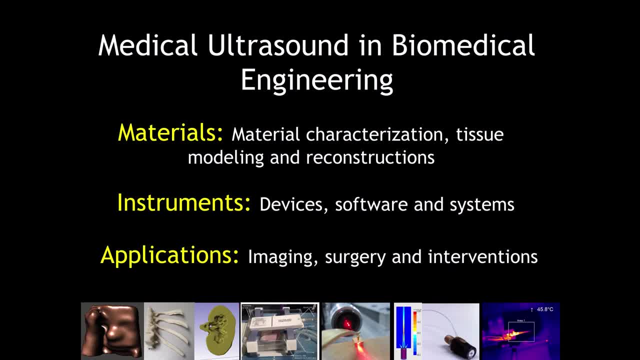 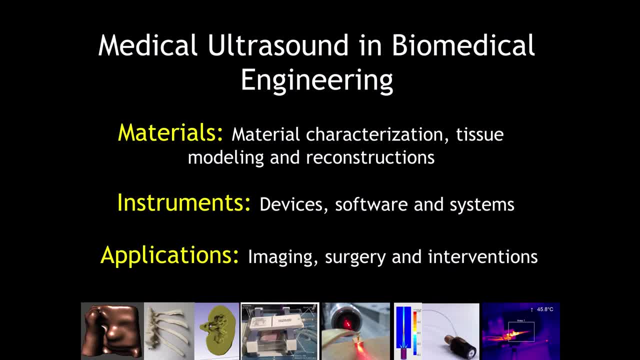 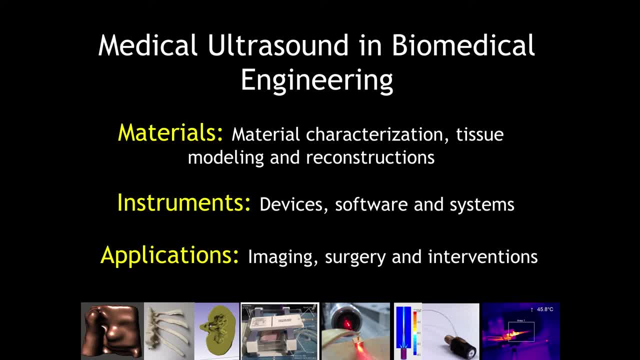 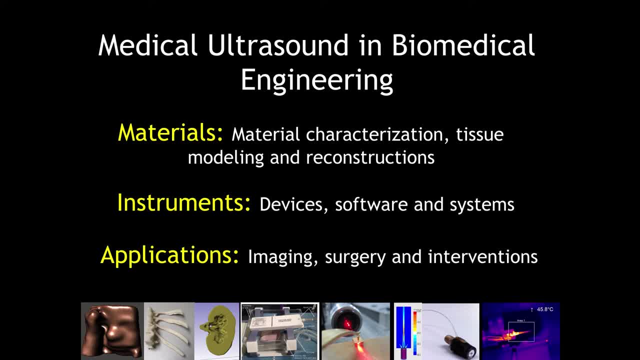 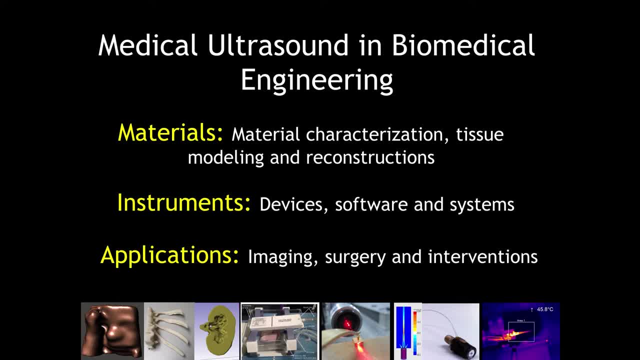 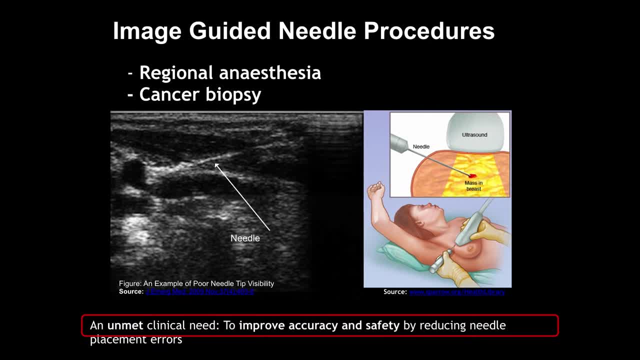 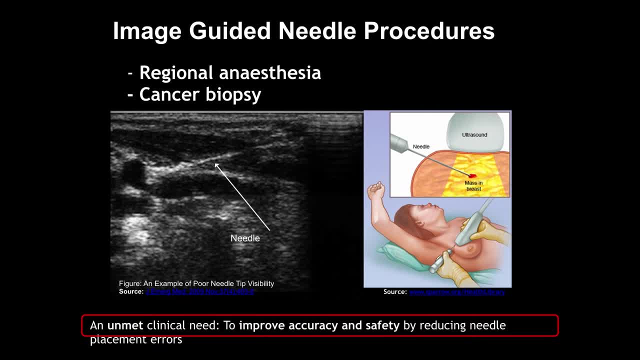 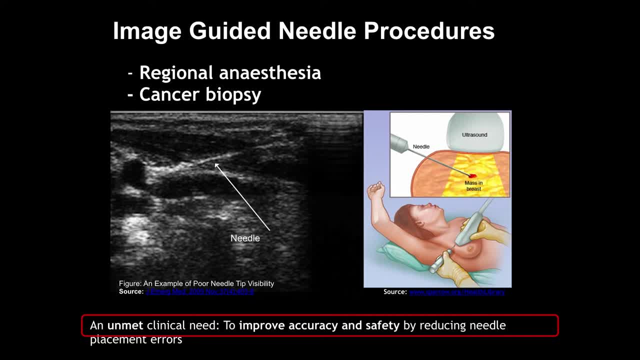 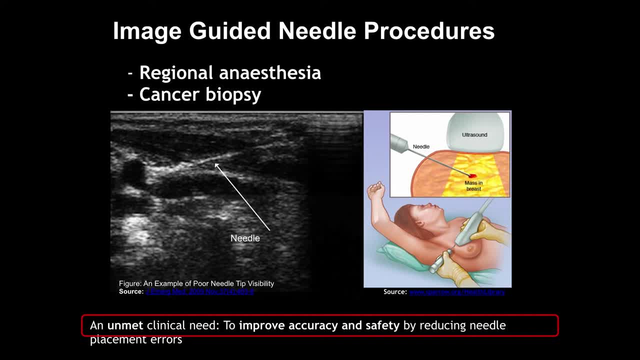 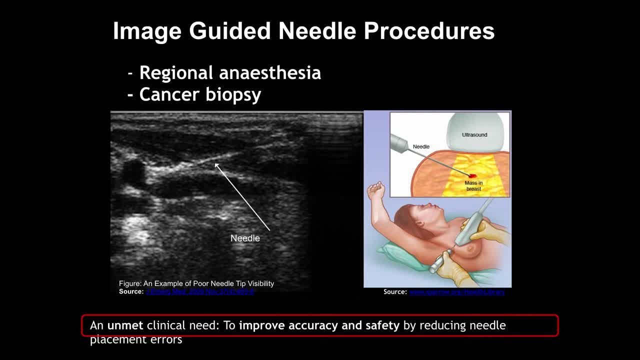 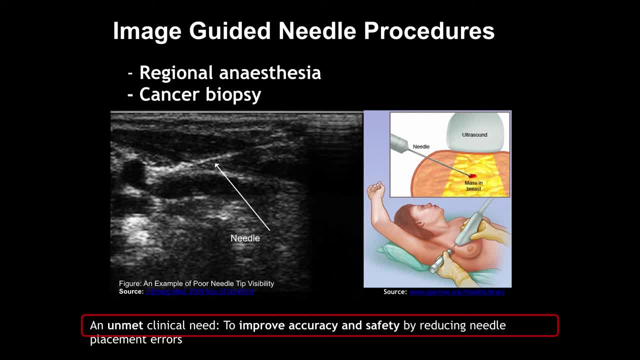 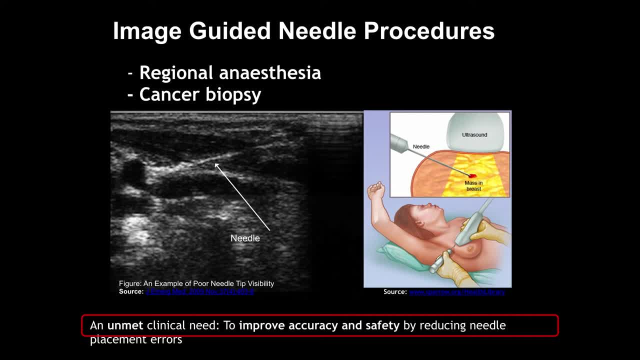 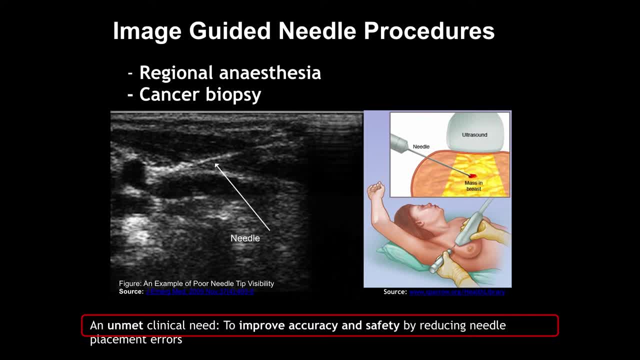 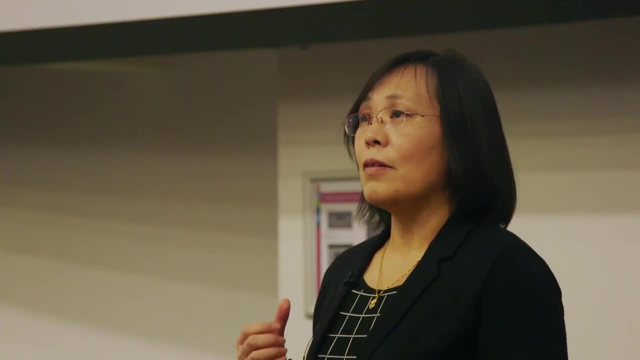 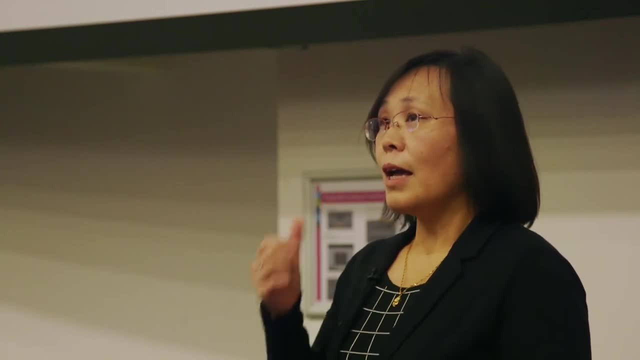 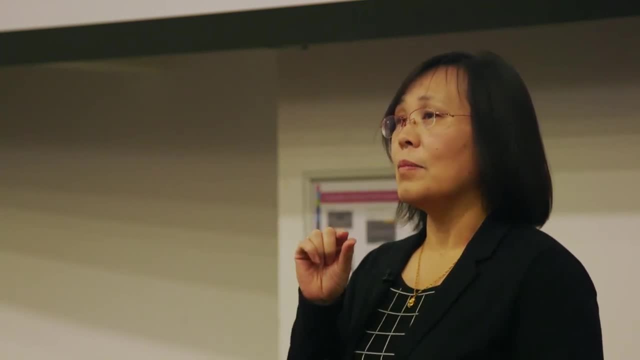 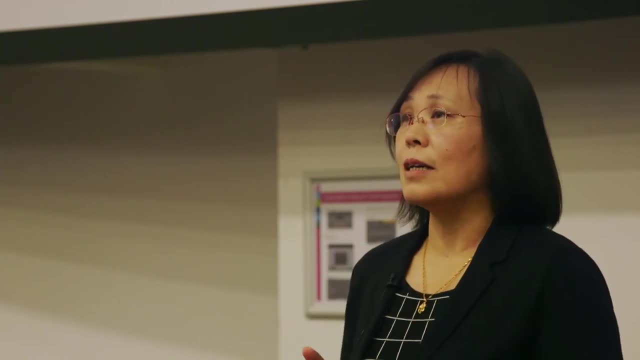 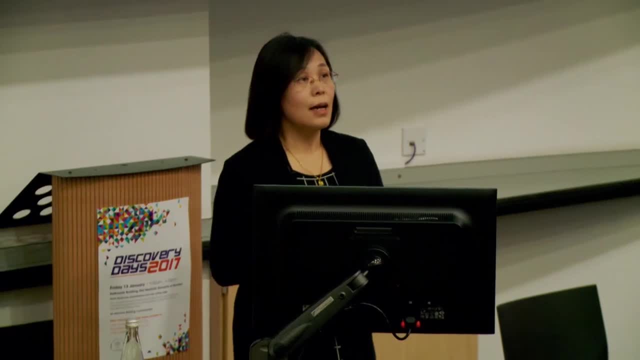 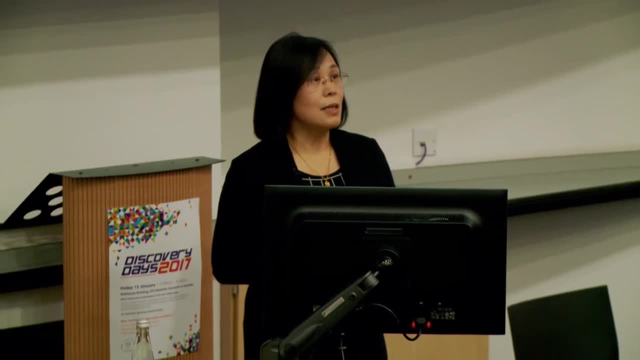 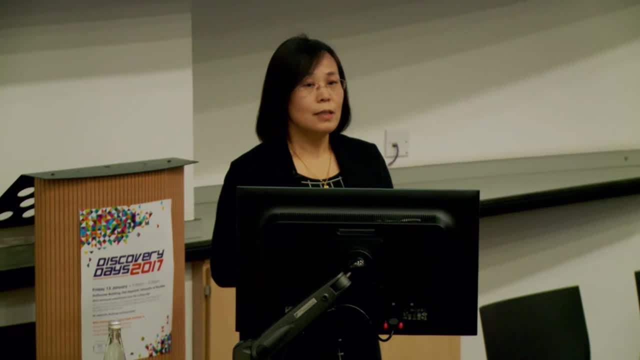 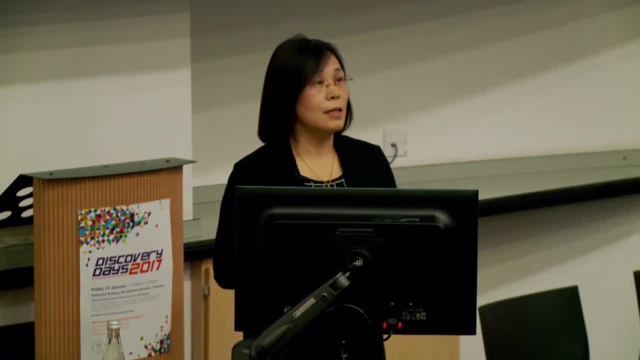 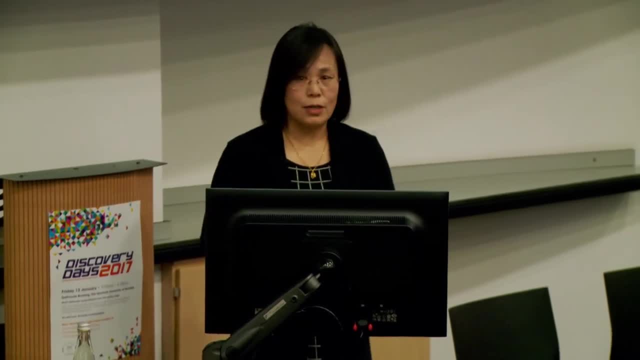 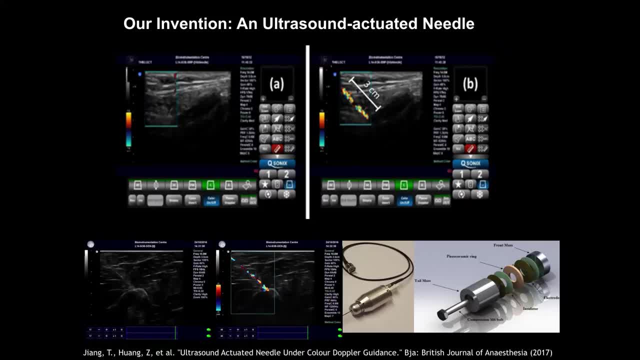 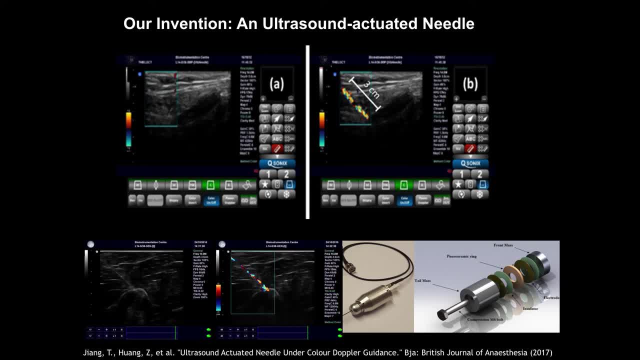 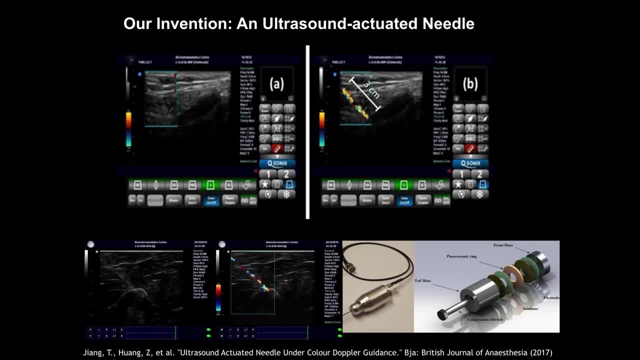 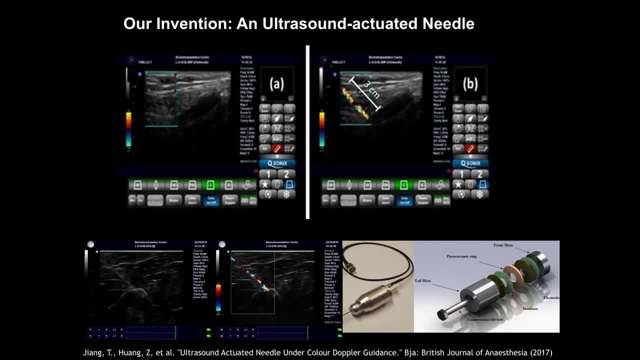 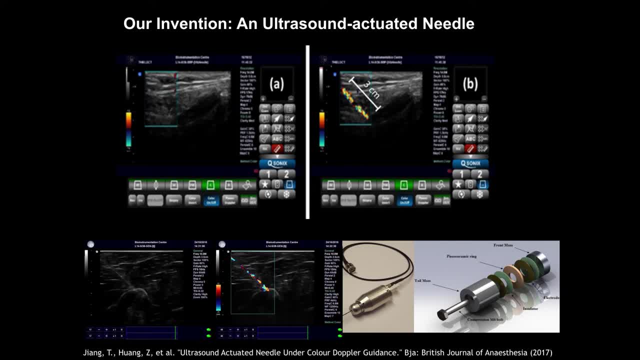 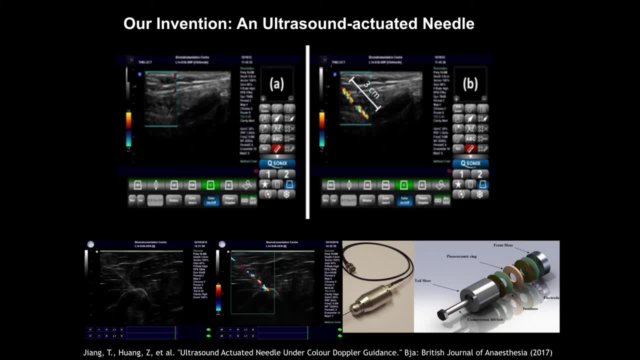 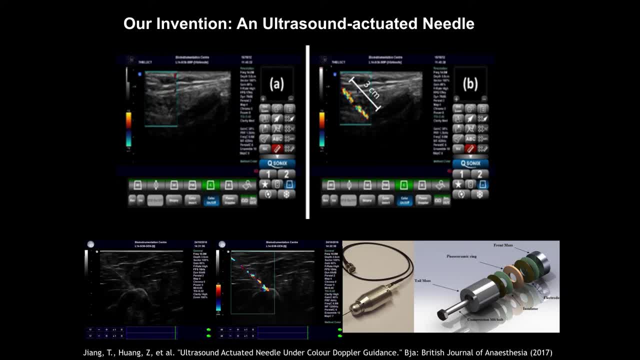 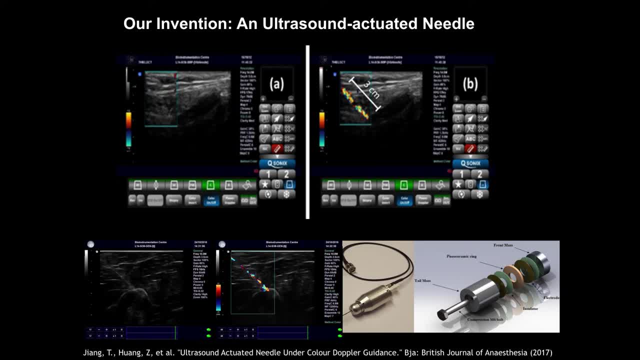 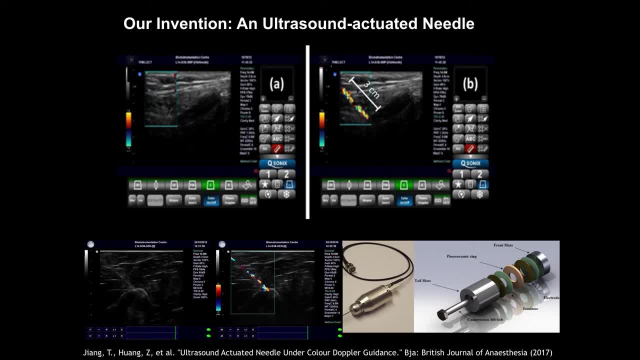 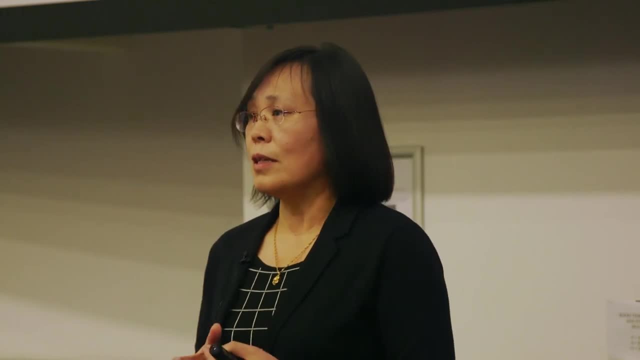 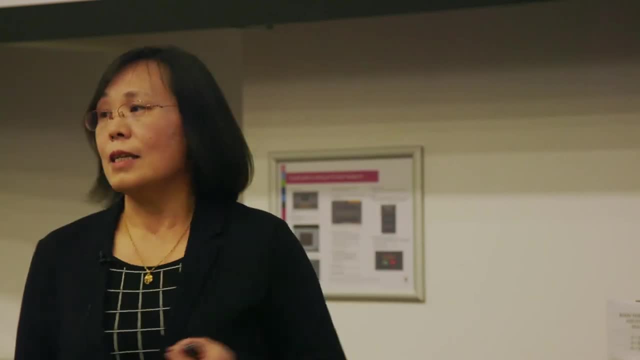 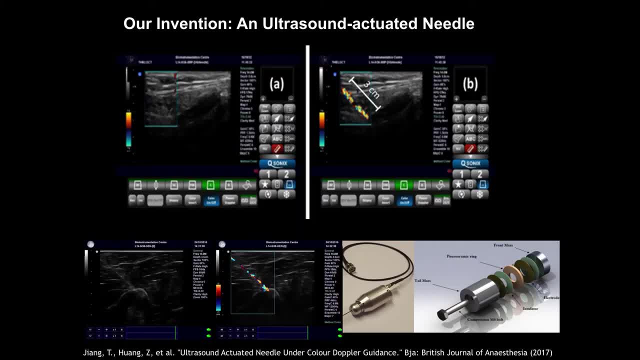 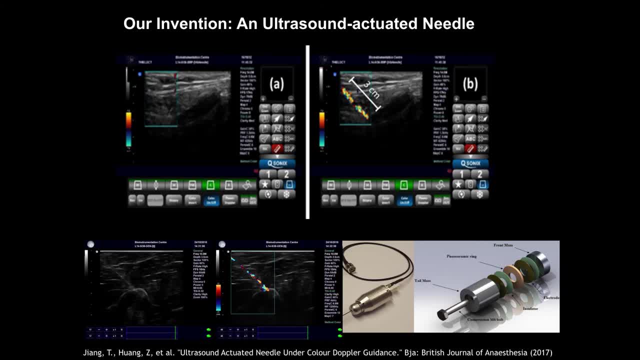 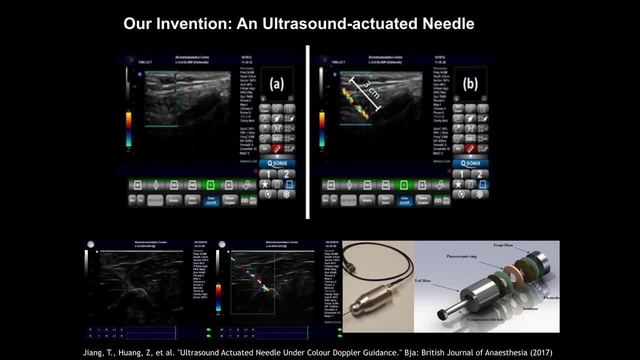 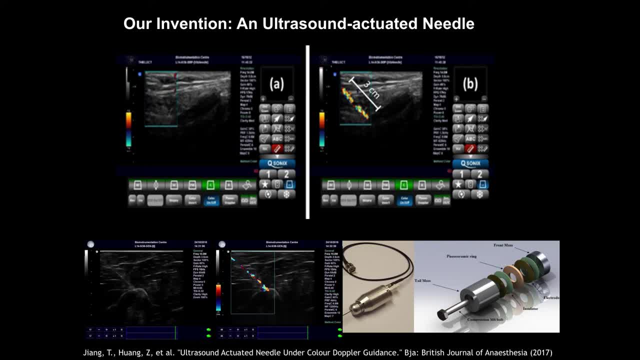 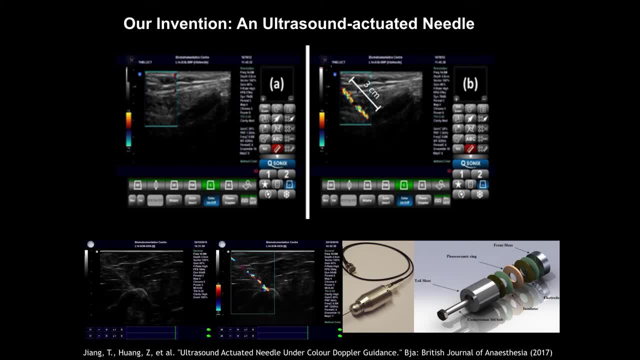 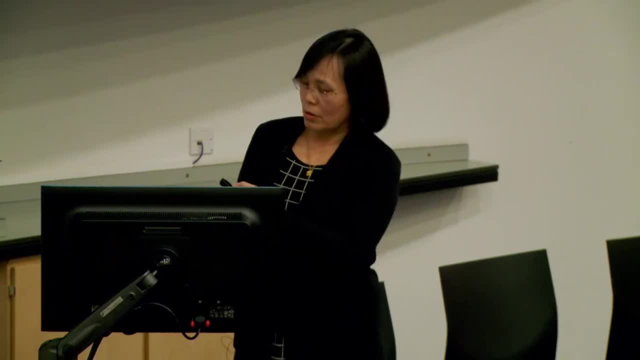 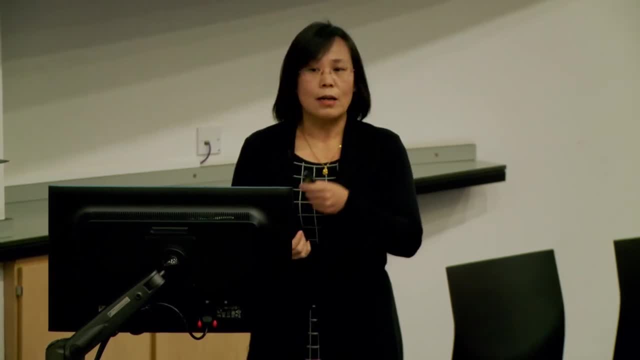 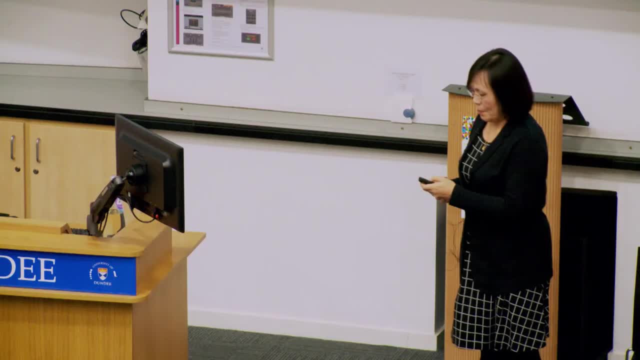 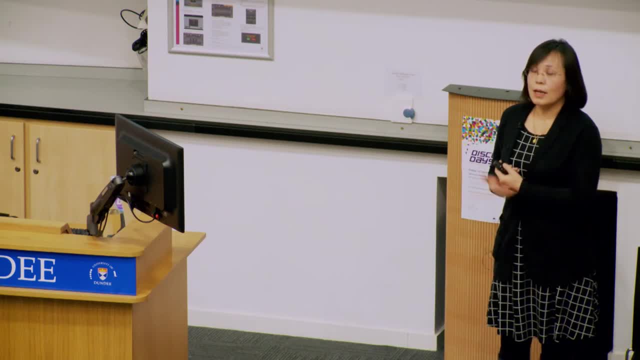 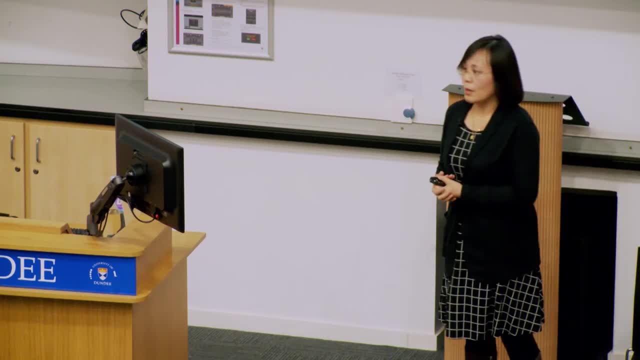 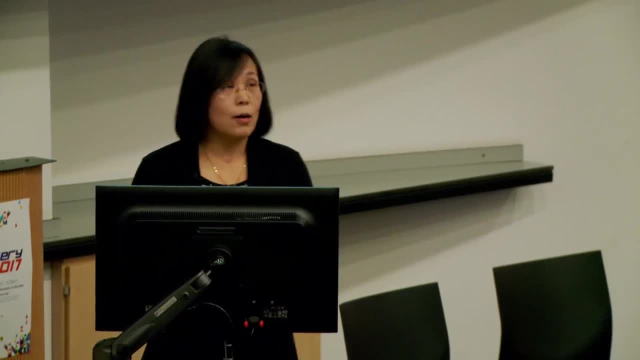 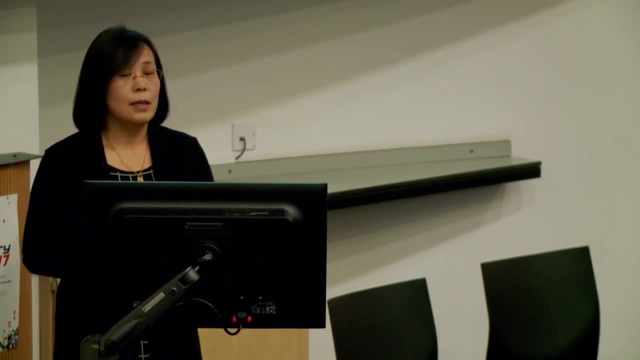 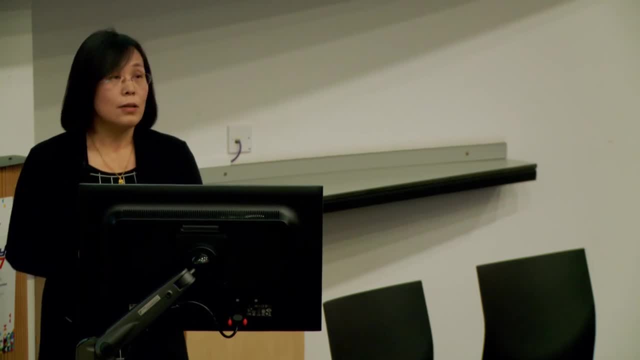 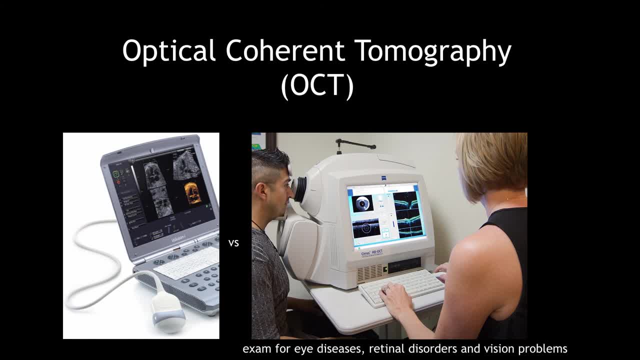 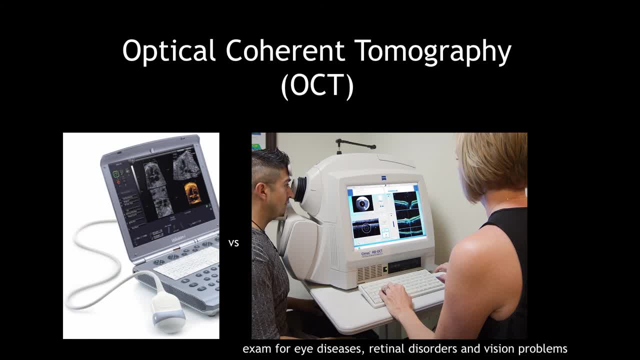 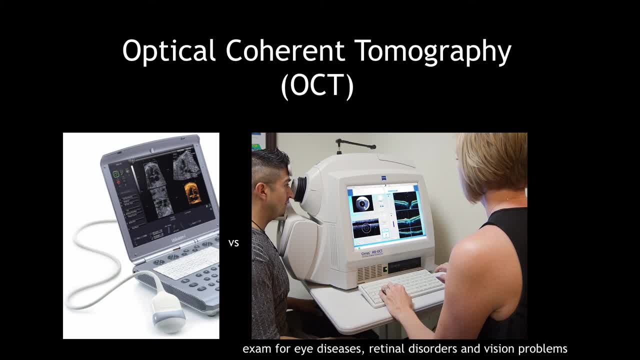 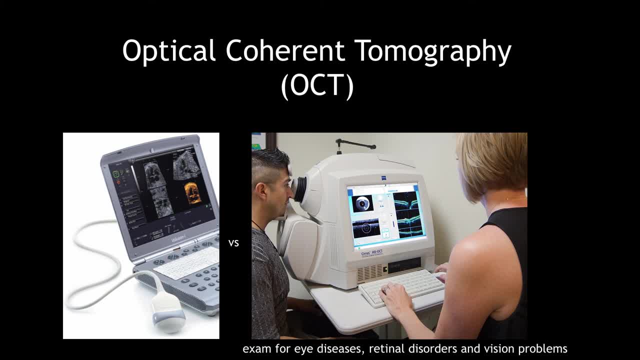 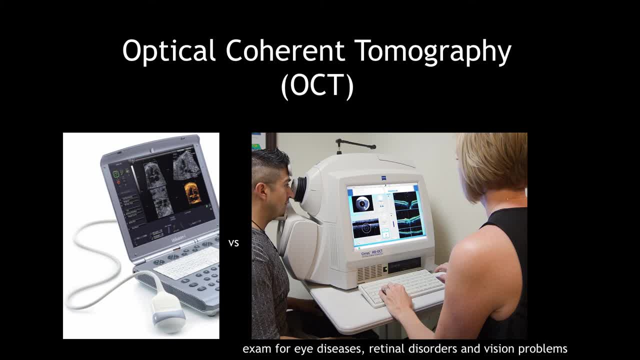 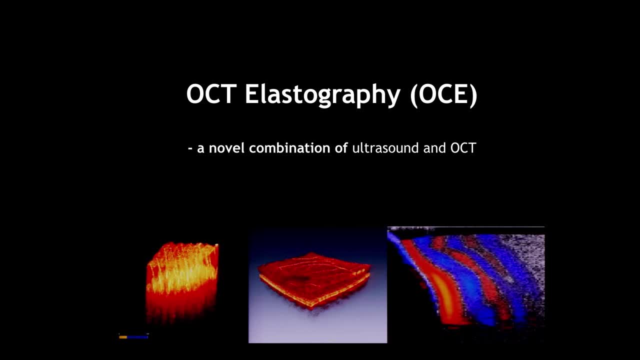 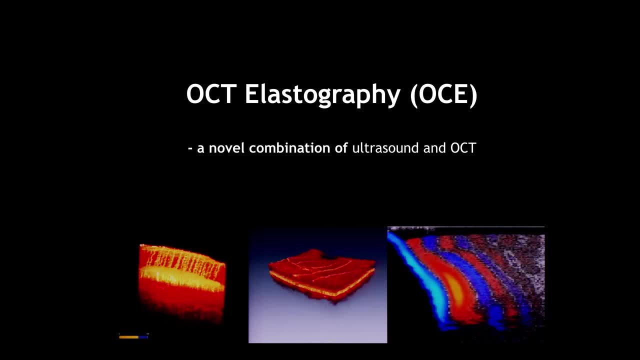 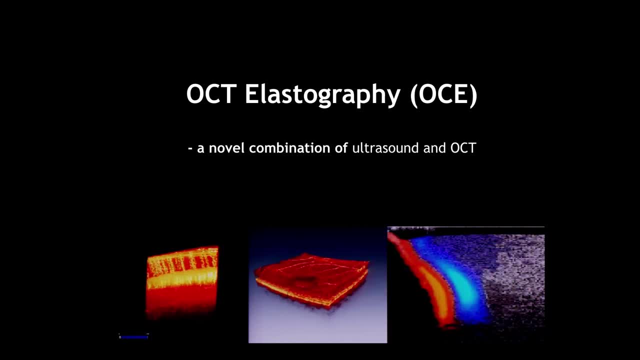 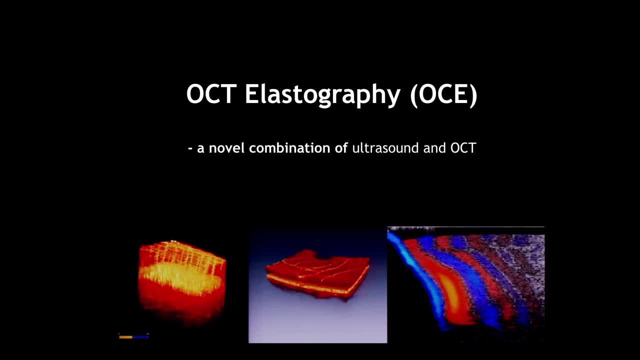 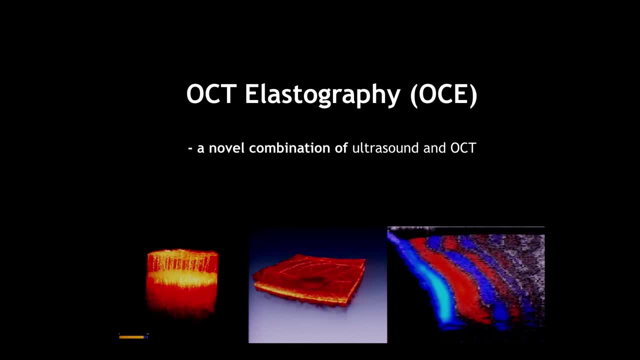 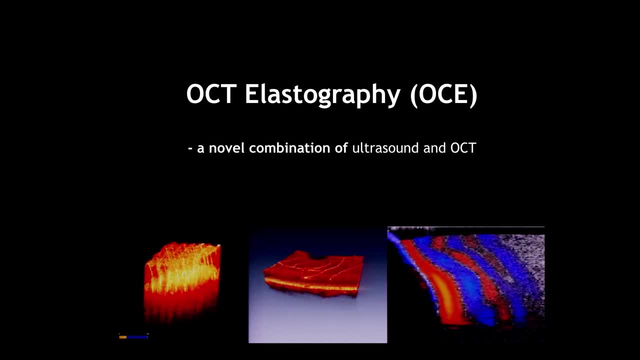 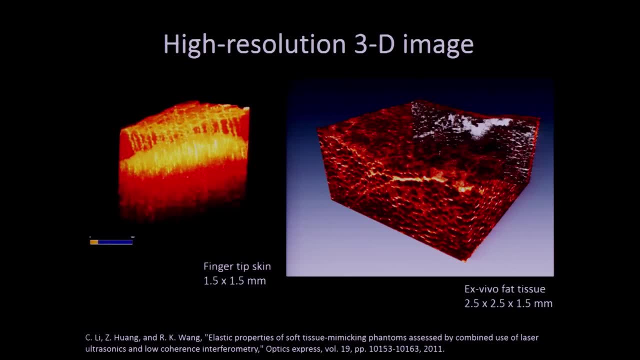 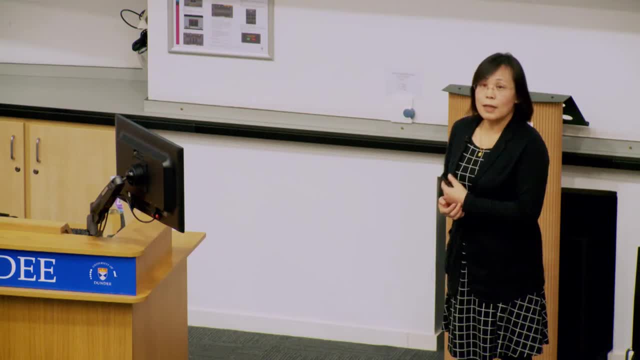 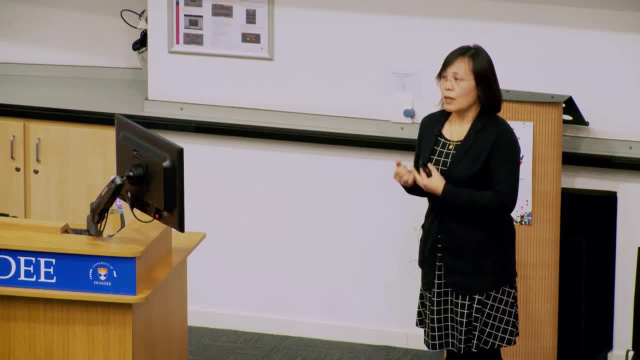 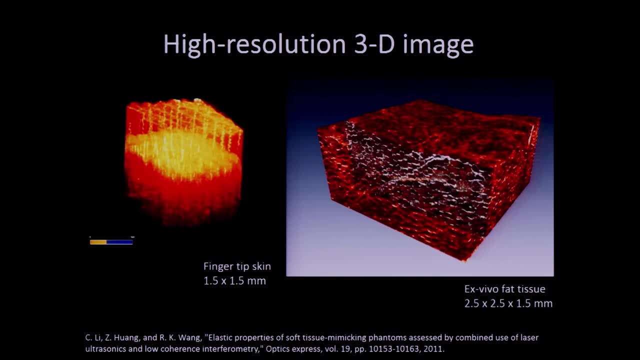 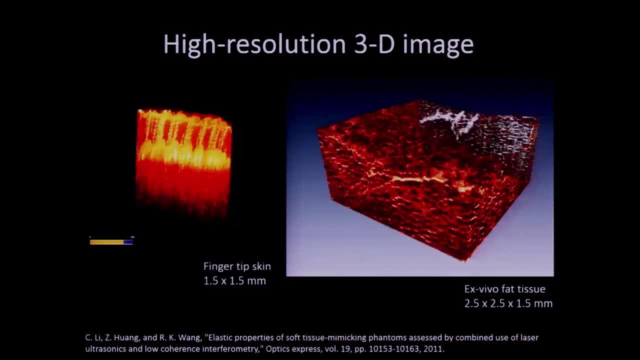 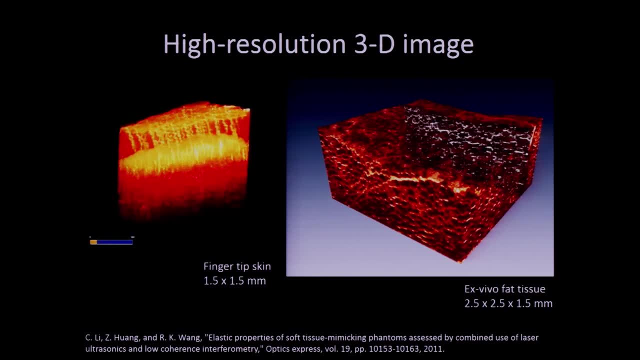 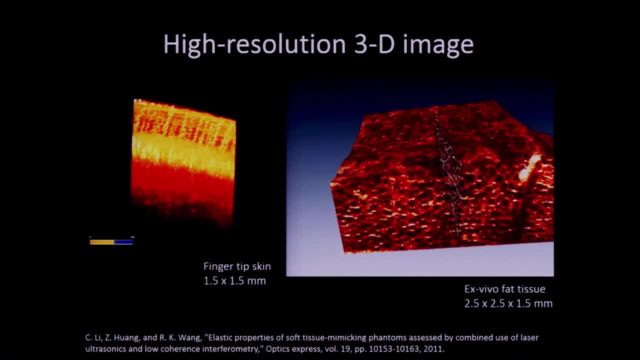 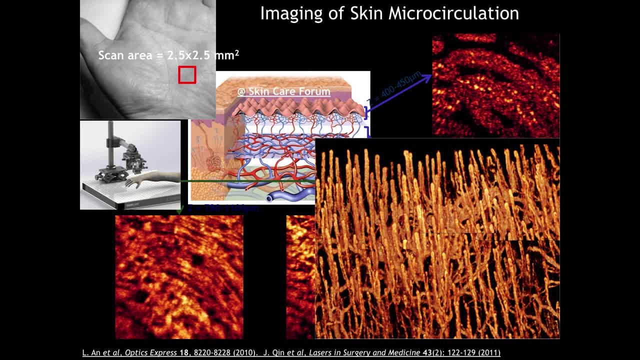 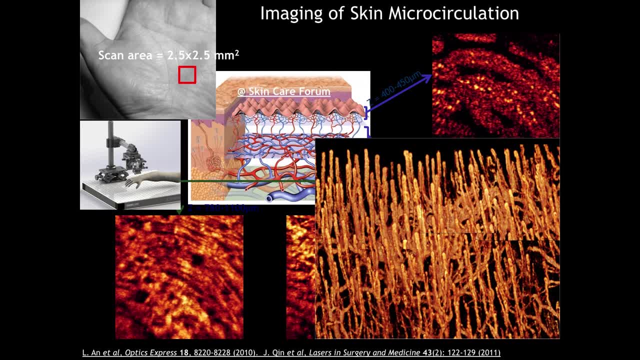 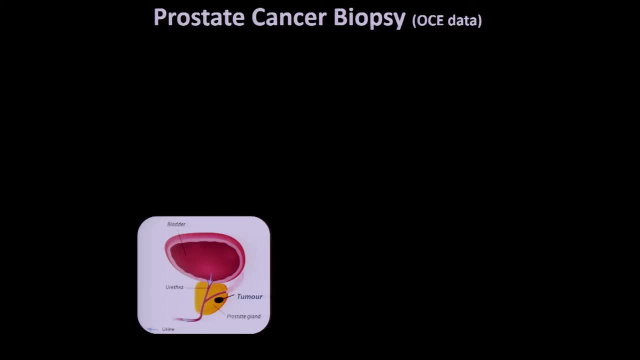 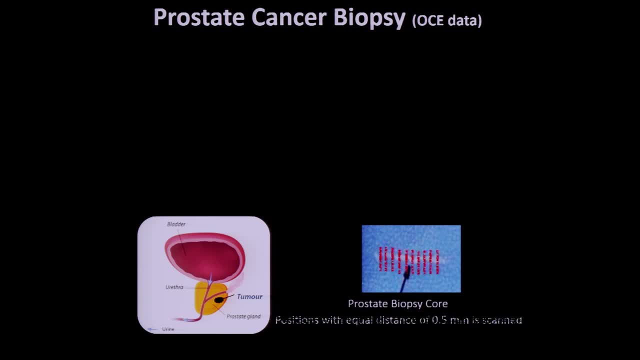 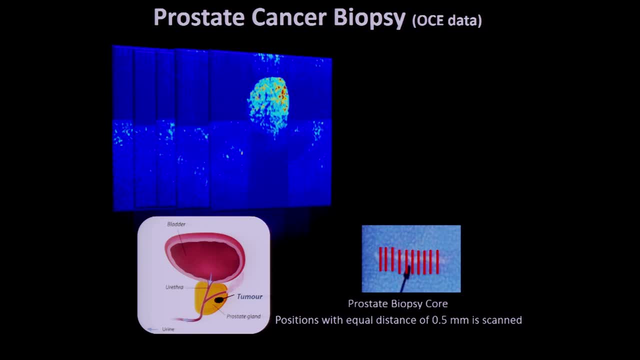 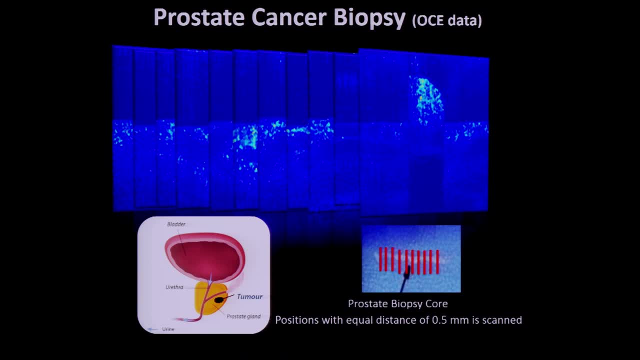 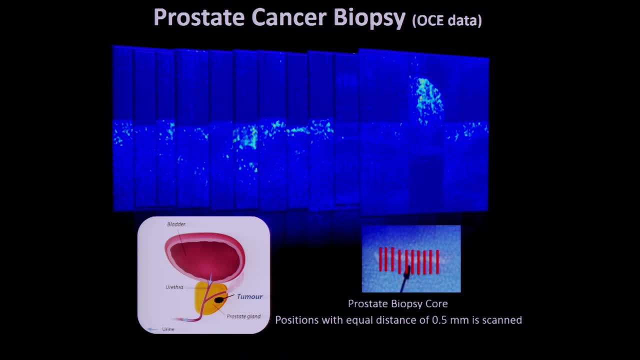 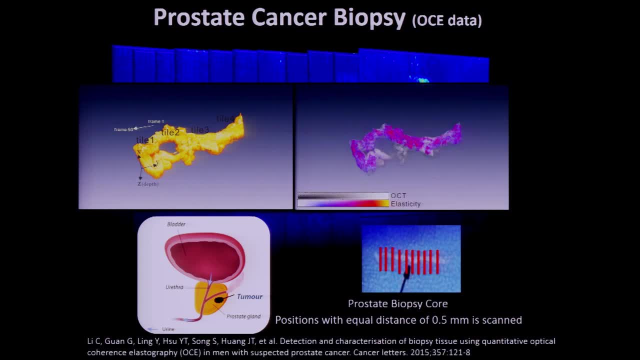 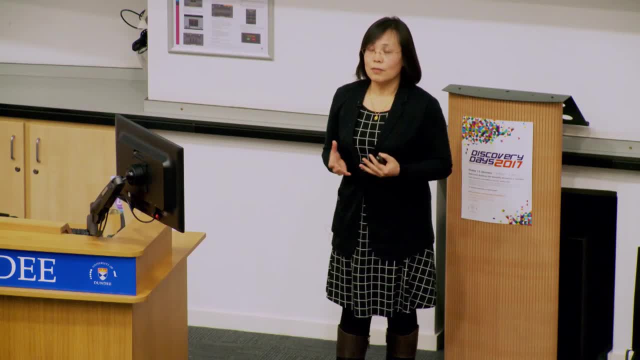 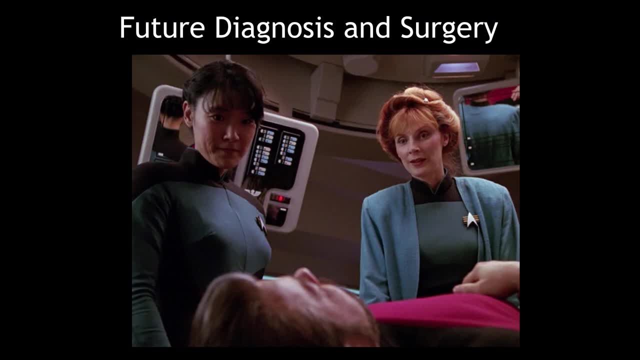 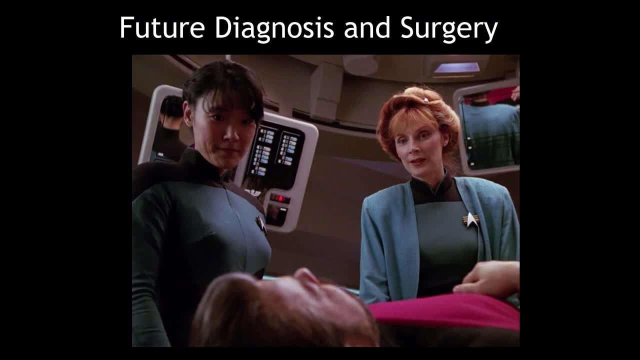 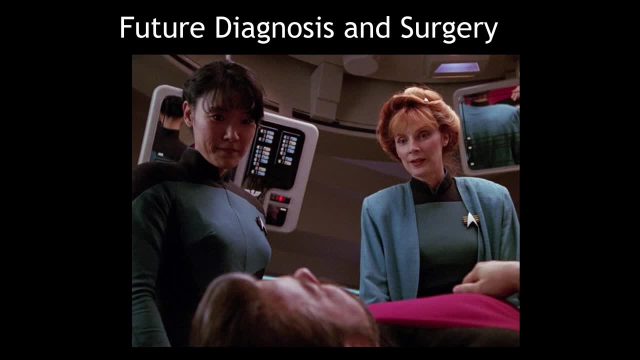 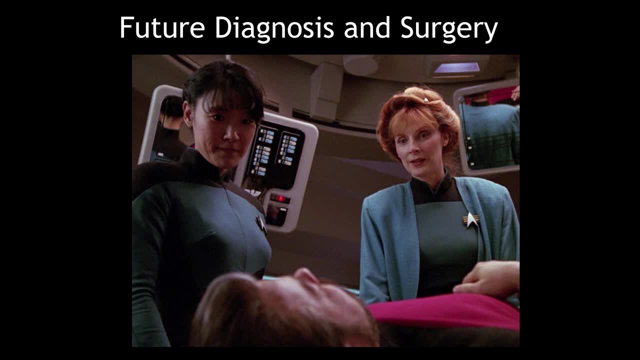 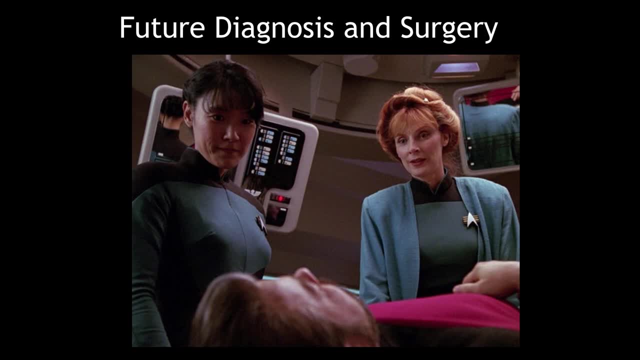 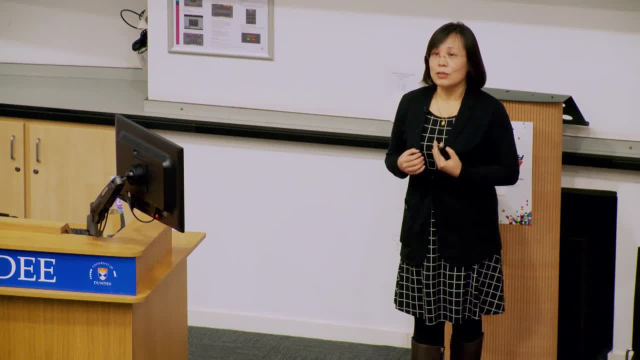 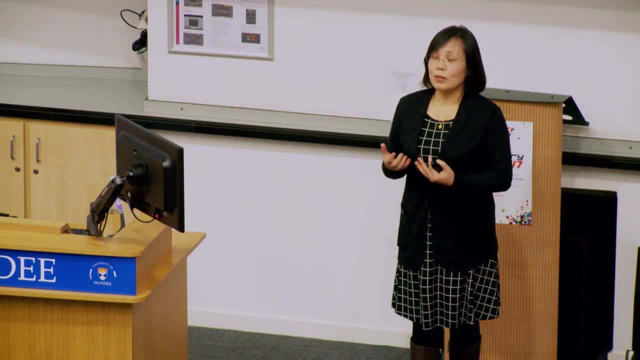 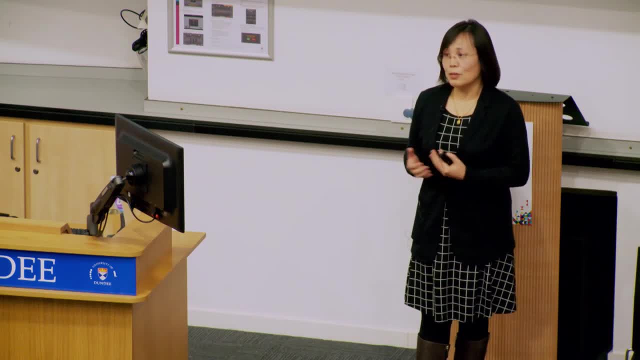 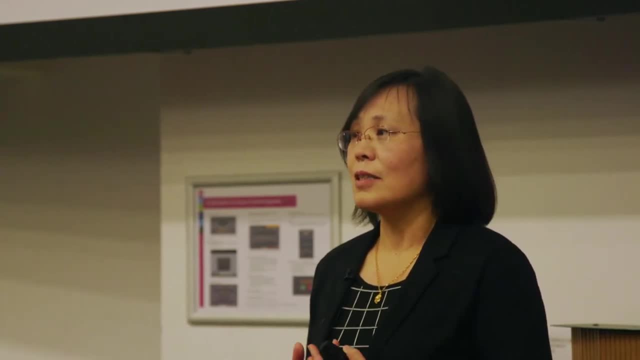 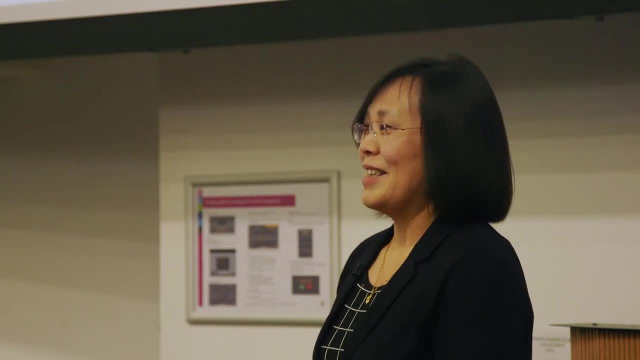 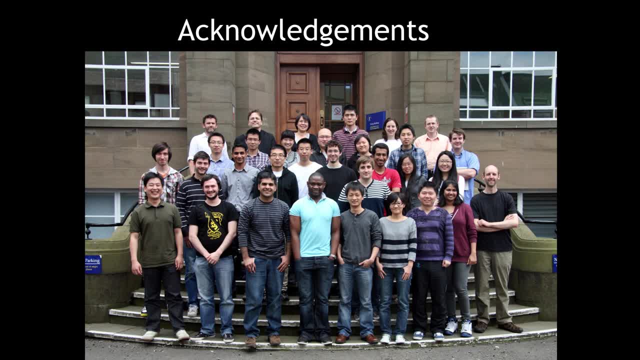 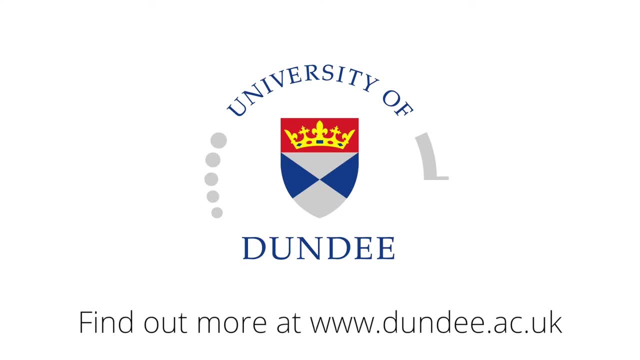 So in our labs over here we develop nice models for ultrasound. So in our labs over here we develop nice models for ultrasound. Thank you, 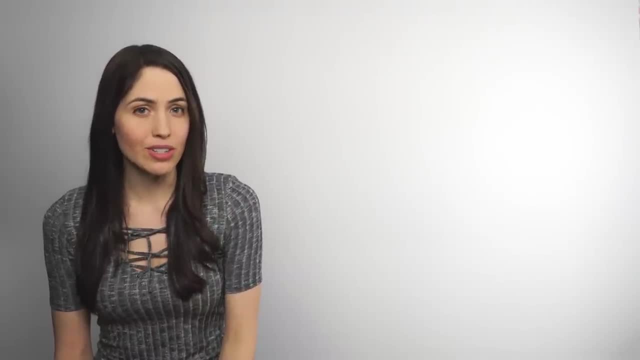 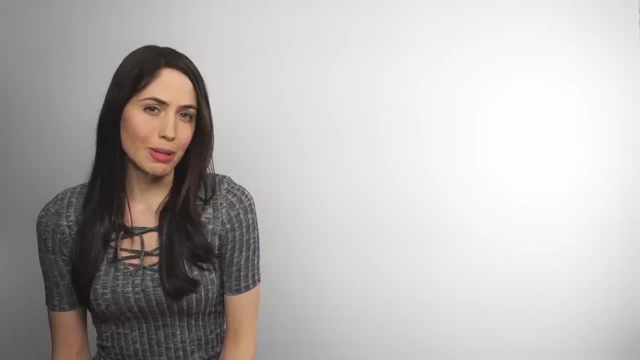 Hi guys, I'm Nancy and I'm going to show you how to use trig substitution to integrate. Listen, guys, trig sub is kind of intense. It's one of those ones where it's probably better to just jump in and figure it out. but don't worry, I'll be right by your side, So let's do it. 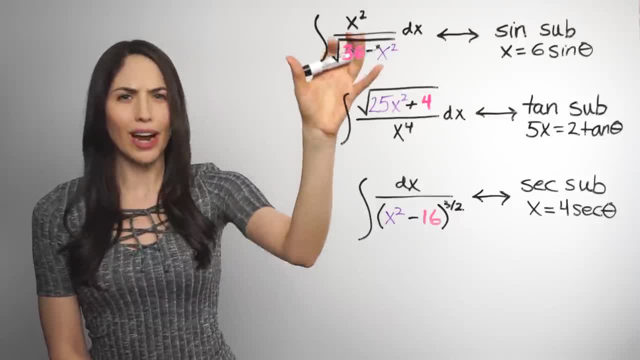 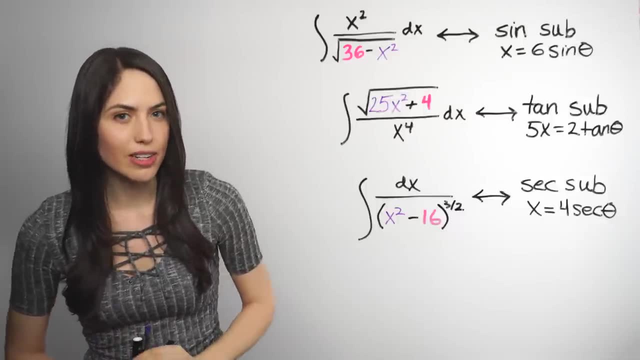 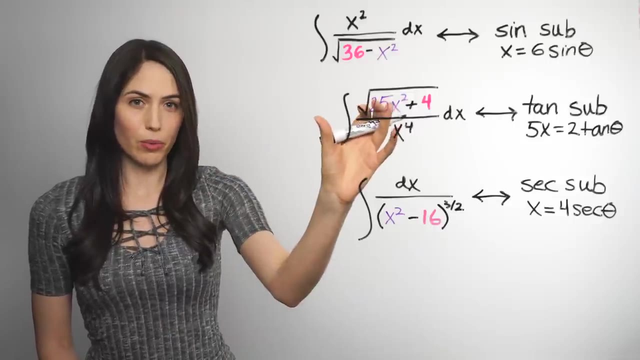 All right. so say you're integrating something that looks like this with a radical in it, and you've tried other things and it's not working. That is a dead giveaway. to try something called trigonometric substitution, or trig sub, as the cool kids say, Basically, lets you get rid of the root. 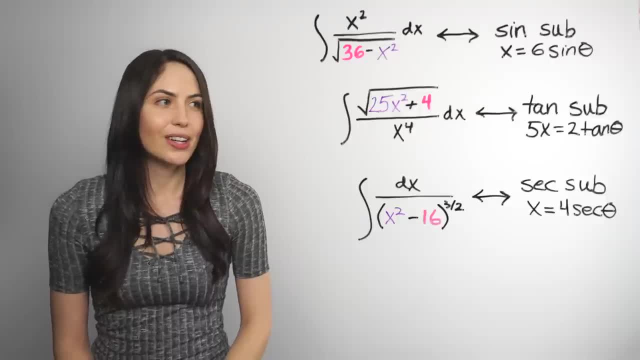 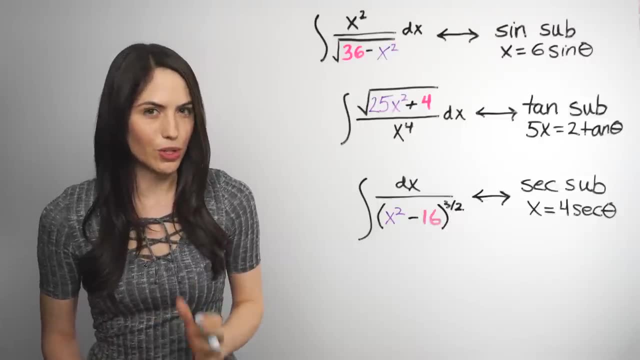 so eliminate the radical so that you can integrate. And what you're really going to want to know is how do you know which kind of trig sub to use, which one to choose? So, in general, if you have a number minus an x squared,